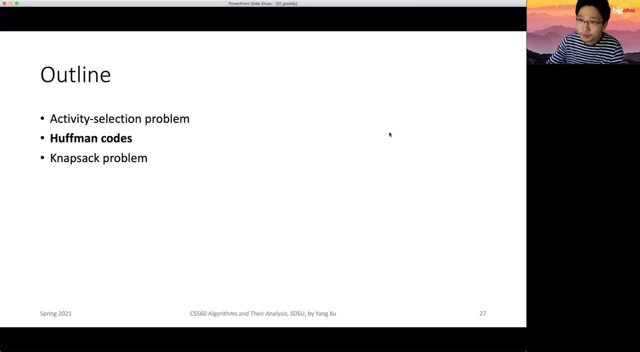 Good morning, Good afternoon actually. So yeah, we're going to continue talking about the greedy algorithms, All right. so last time we have finished the activity selection problem And today we will look at the next two types of problems. 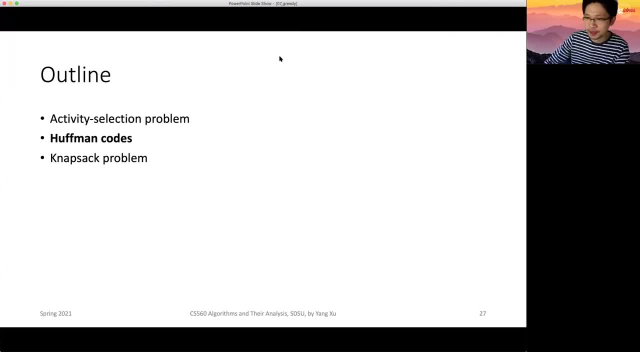 Huffman codes and knapsack problem. Okay, So these are very typical problems that can be solved using a greedy algorithms. Well, in fact, when the solutions for these problems are first invented, I don't think people will like realize that, okay, this is a greedy solution, but it's a greedy algorithm, is just a. 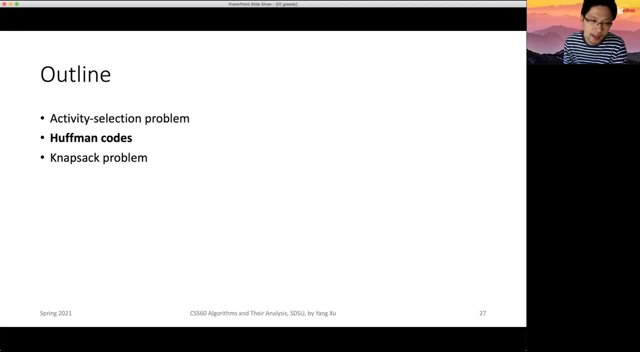 way to summarize the common places of the algorithms adopted in these problems. Okay, so let's look at the Huffman codes first. All right, And so in practice, it's a very commonly used algorithm for data compression. Okay, So the codes here actually. 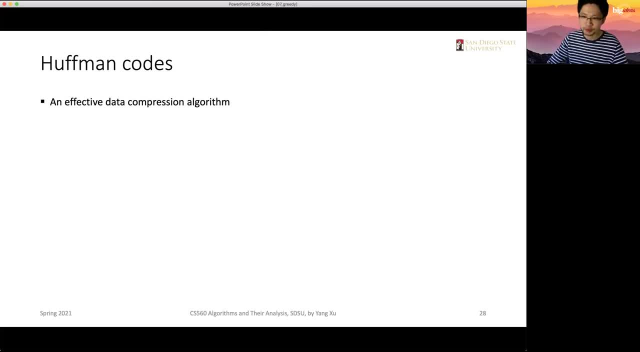 refers to process of encoding data, like encoding string data or basically any kind of data, into a compact binary format. So in this example that we use here, the data is actually a sequence of characters and our task is to basically represent each character using a binary code. 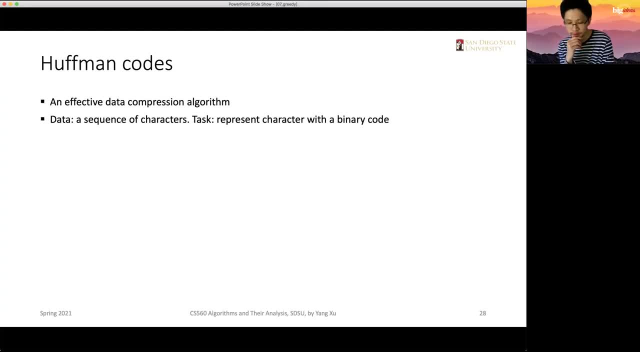 So this is also a very common scenario in natural language processing- that when we want to input a bulk of text into the machine learning models, like, we basically need to first represent this text as a sequence of characters, And the most efficient way to store and retrieve this sequence of characters is that we 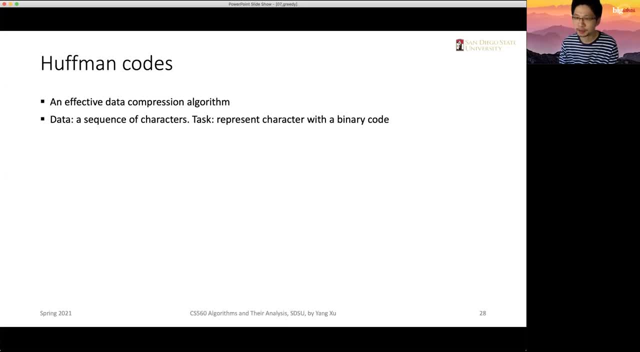 want to encode them into a binary format that is efficient, memory-wise, memory usage-wise. Okay, So the basic principle is that we need to use the frequencies, use the frequency information- basically, it's a table of character frequency- and then we use that to represent each character as a binary string. 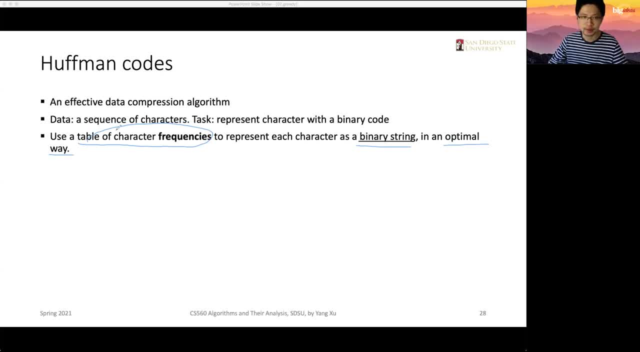 Okay, so hopefully to optimize the way of encoding so that as few memory space is used as possible. Okay, so for example, in this table, like we use a rather small vocabulary and we assume that there's only six unique letters or characters in our data, Okay, we only have from A to F. Okay, 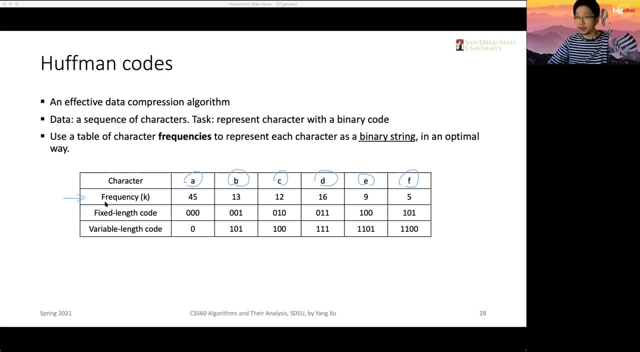 and also the second row. it shows the amount of our data sets. It counts how many times the letter, the character A, has appeared. For example, in this case, the letter K, the A has appeared for 45,000 times and less for B, which is 13,000 times, and so on. 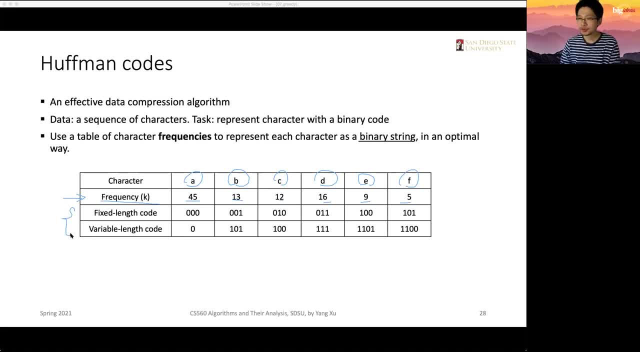 So next, in the next rows here, we show two ways to encode the letters in a binary string. Okay, the first is called a fixed length. So, as the name indicates for each character, we will encode them with a code that has the same. 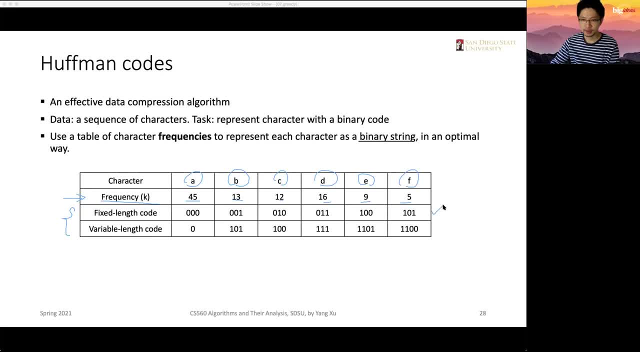 length with fixed length, And it's three binary digits, right, with three digits. So for A we use 000, and for B we use 001.. So it's just like a binary number, right. We increment this encoding by one for each character. Okay, so this is a so-called fixed. 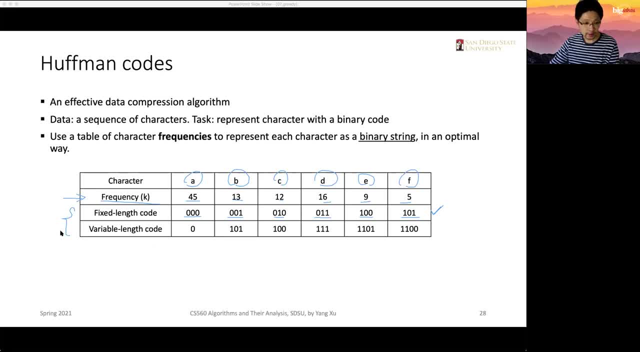 length code And, on the other hand, the second row, the variable length code, is actually our focus today. Okay, so we will use a different length for different characters. Okay, and you can see that the letter A has just one digit. Okay, it's just one bit. Okay, so this one bit. 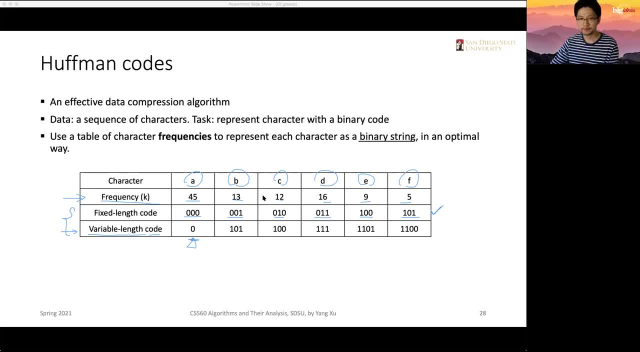 either 0 or 1, we use 0 to indicate this is A, and for B, we will have 101. And for C, we have 100.. And for the E and F we use four digits. Okay, you see the difference here. 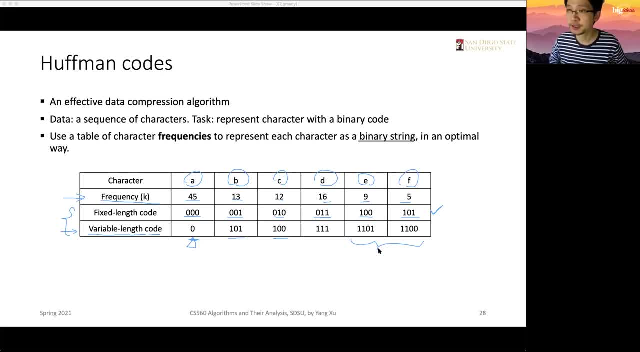 We use different lengths for characters with different frequencies. Okay, so maybe the intuition already tells us that. okay, this might be a better way, because the character A is the most frequent letter in our data. so it makes sense that we use less memory space, we use less code to encode the most frequent one. 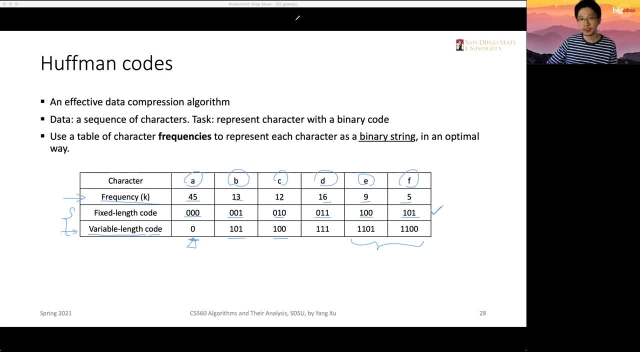 So this is a very smart principle and let's basically check out how we achieve this, how we implement this algorithm in an efficient and in a valid way. If we simply count how many number of bits needed for different ways of encoding, one bit is for just one digit here, so this one digit is one bit. 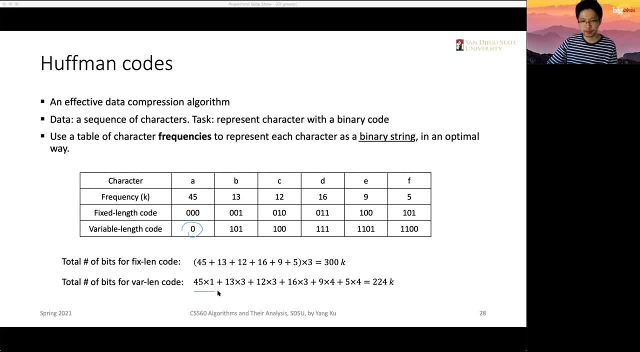 For the variable length it's 45 times 1, right, because A appears 45,000 times, so it'll be 45 times 1, and for B it will be 3 times 13,, because it appeared 13,000 times and each time we need to use 3 bits. 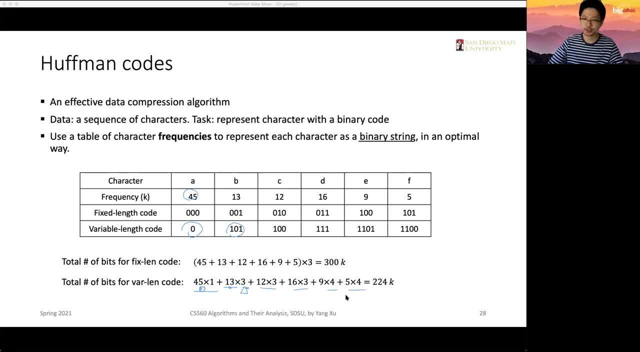 and so on. So, for all the letters, we can use the summation of these products to calculate the total number of bits required using this encoding schema. All right, so the difference is there. Obviously, the variable length code is better. right, because it uses less bits. okay, because bits is the way to quantify. 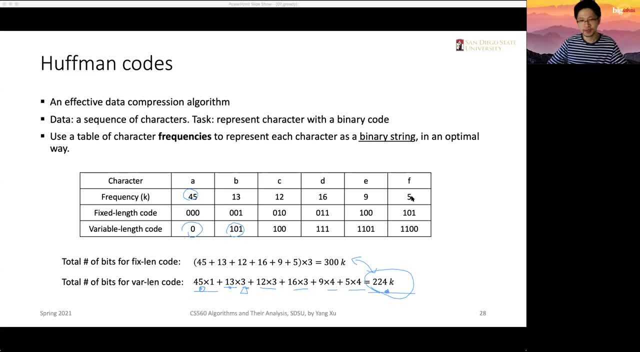 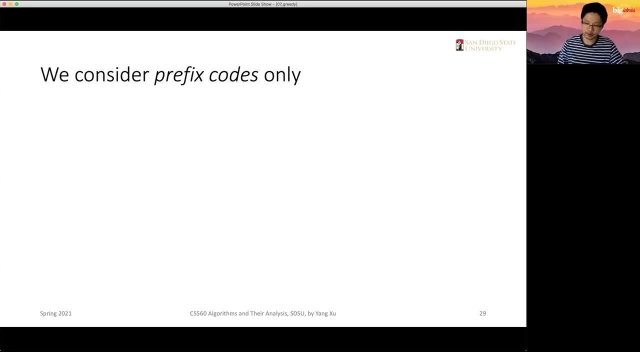 the amount of information required. right, so this is an obvious advantage of this variable length encoding. So, for using the variable length encoding, there's a technical issue we need to pay attention to, which is that these particular codes, variable length codes- need to be a prefix code. okay, So? 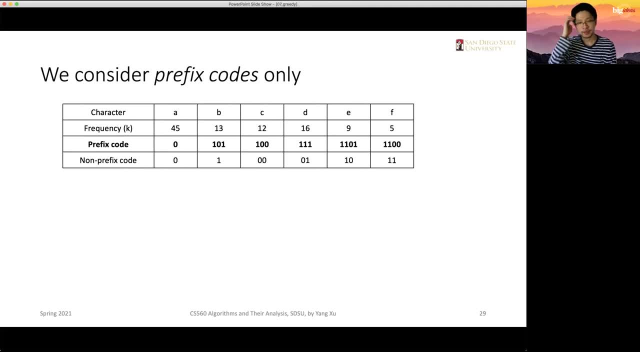 this prefix code is a property that makes sure no code is a prefix of some other code. okay, So if a one code is the prefix of the other code, then it causes ambiguity when we decode, In the decoding stage, For instance, if we encounter the binary sequence like this, which is: 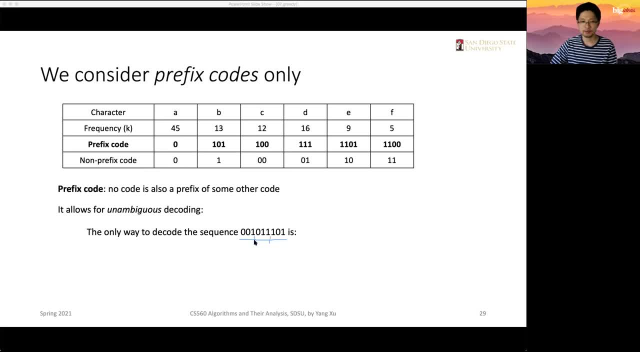 001, 011 and 10.. one right. so how do we decode this sequence according to the the table? right? we have two ways of decoding, right? so if it's the prefix code, then we can. when we first meet the first zero right, the table will tell us: okay, this is a letter a. and then when we meet the second zero, 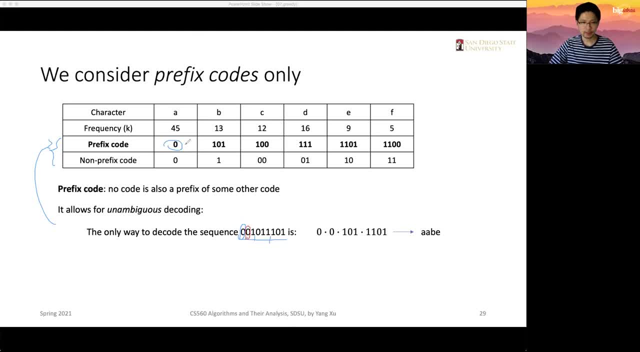 it's another zero right, then the table will tell us it's a again right. and when we meet a one, then the next three letters is: oops, is 101 right, right, so 101 would be so if we decode this sequence, use the prefix code encoding. 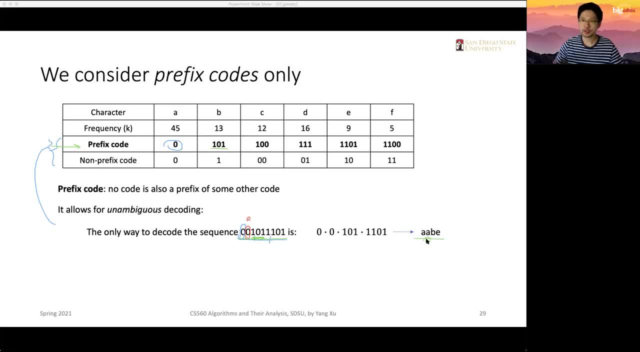 uh, schema, it will be a, a, b, e, right, there's no ambiguity at all. but it will be not the case if we use the non-prefix code. which is that? okay, you see, the um, the, the, the encode, the. the code for a is zero, right, but the code zero itself is the prefix for c, right, it's also the prefix. 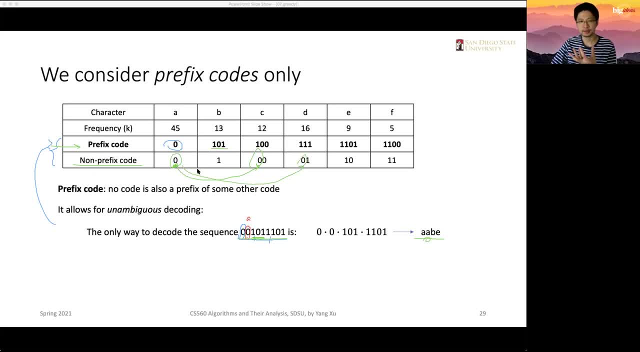 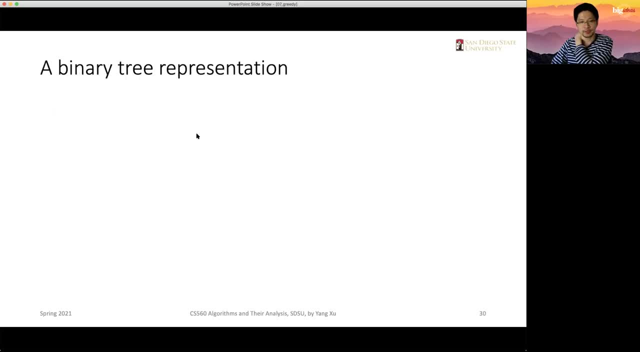 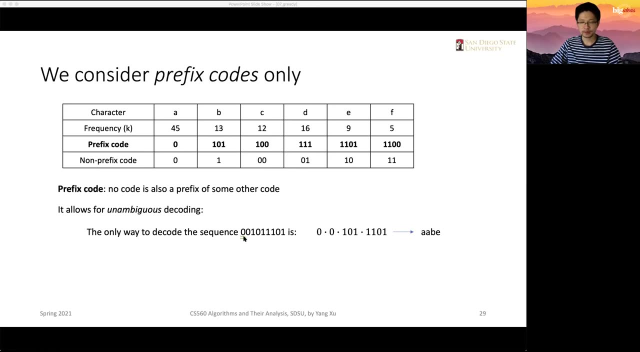 for the d here zero has appeared at uh, as the first letter in these three encodings. so this causes trouble for us. so, like for the same sequence if we look at the first digits, right. so there's two ways, two different ways to interpret right. it could be either an, a right, or it could be the two consecutive zeros, which corresponds to. 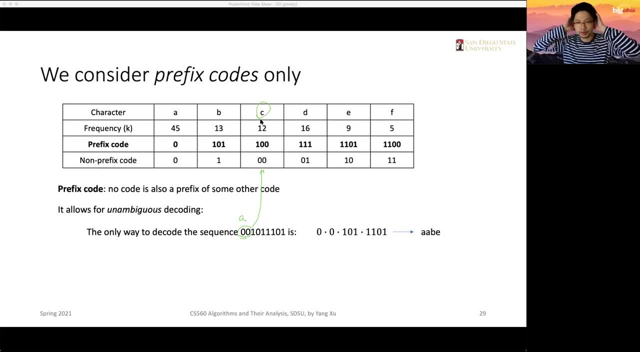 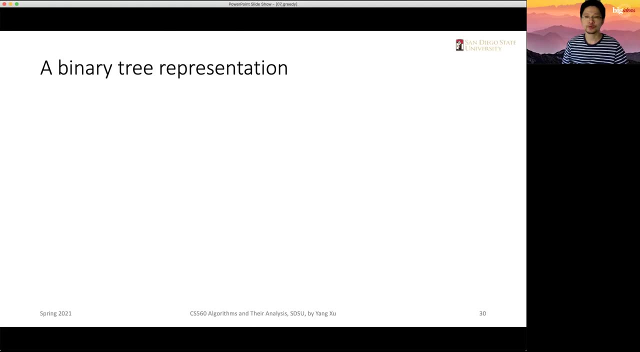 the code for c. so this is definitely what we uh, uh, uh don't want, right? we want to a unambiguous uh, decoding and encoding. okay, all right. so basically our task is to to get a uh and then design the algorithm to to uh efficiently encode each letter according to their frequency, so that the, the codes are. 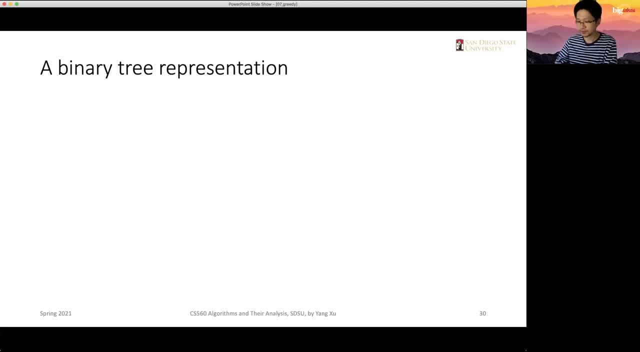 variable lengths and, more importantly, they are prefix codes. okay, anyway. so the data structure we're going to use is to uh, uh is is a binary tree, okay, so a binary tree can provide actually a very convenient uh representations for the prefix codes. okay, and in the tree we will have leaf nodes and non-leaf nodes, so the leaves, in this case, which are 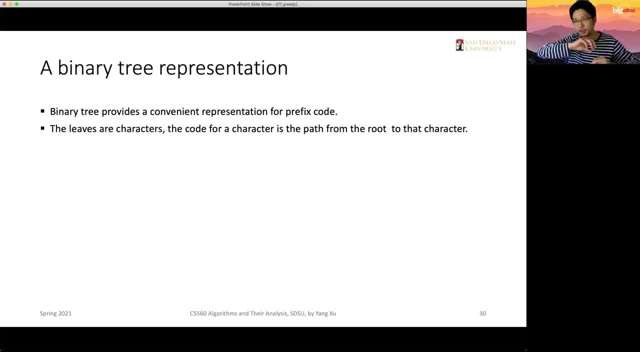 are the most uh bottom nodes that do not have uh children nodes. those leaf nodes are characters, okay, and the code for capture is the path from the root to that character, okay. so, for example, this is a binary tree that that is already encoded, it's already uh built, okay, or drawn, so this tree is complete. so if we look at the binary, 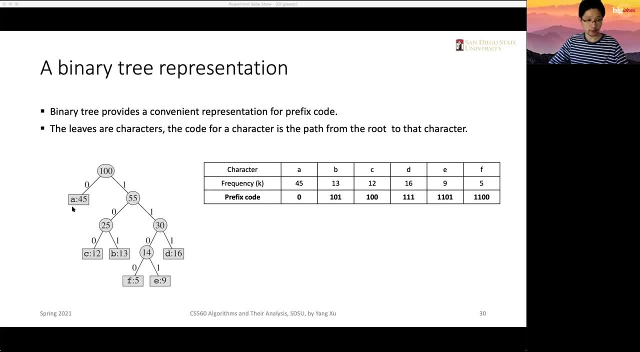 uh, if look at the leaf nodes, they are all in these, uh boxes, okay, on these rectangles. okay, so i, we also attach the frequencies to that letter, right? just for information, just for showcase how the a has the shortest path, right? so if you look at the path for a from the root, 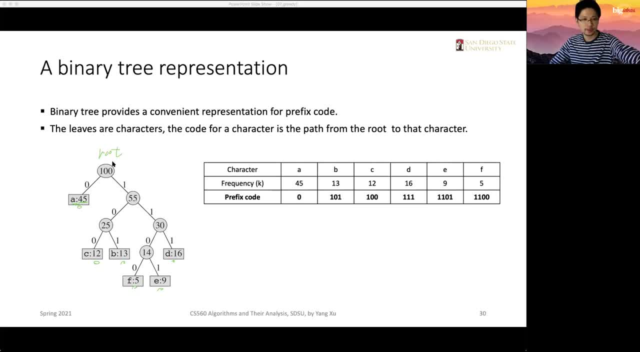 so this top node is the root node. if we go through the a to the root node, we will have just one digit, which is zero. okay, and this zero is exactly the prefix code for the letter a, a and for c. right, if we look at c, it's right here. if we go and we need to go from the roots, 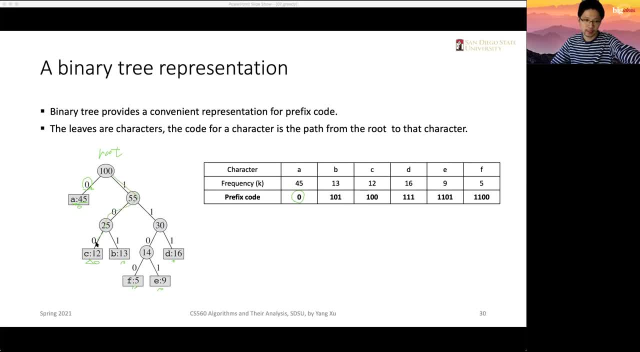 to the c to find its path and along this path, we will have zero, one zero and zero right, which is exactly the code for c and similarly for b right. it's one zero, one right and for the all the other, uh. for the other uh characters. okay, so this is the way we're going to use to uh represent the. 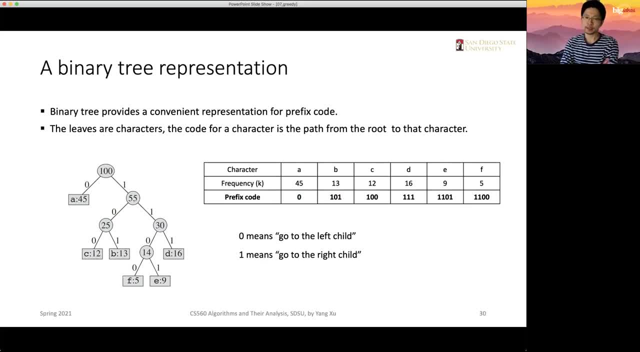 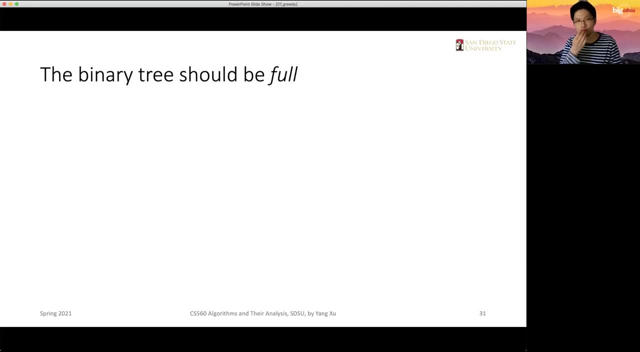 the, uh, the encodes for you represent the code, the prefix codes. okay, so the zero and ones means that this is the: if it's a zero, then we go to the left child, and if it's one, we go to the right child, and this is very clearly defined here. okay, all right so. 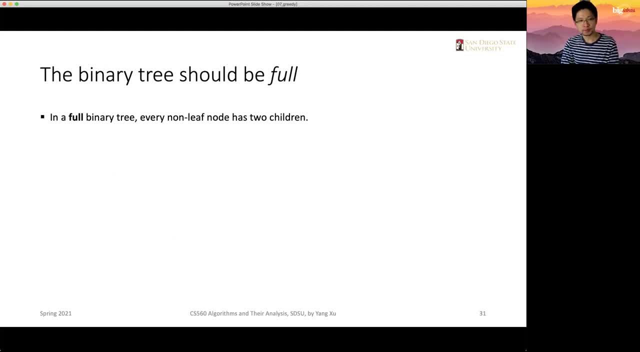 you, um, the binary tree should be a full tree, which means, uh, every node in the middle, which means they are not leaf, every non-leaf nodes, should have two children, okay. there shouldn't be a left and there shouldn't be a an empty branch, okay. so the tree, uh, corresponding to the fixed length. 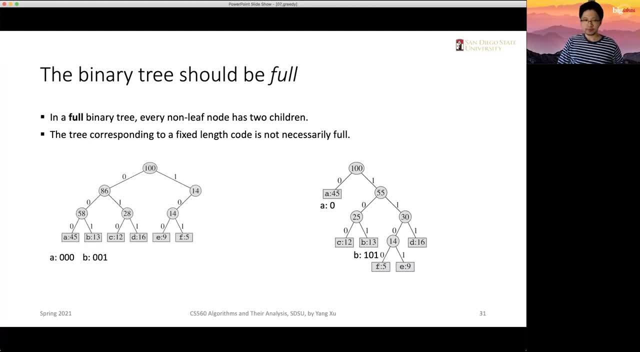 code is not necessarily full. so you will see that, uh, if we compare it with the uh, the variable lens the code which is here right. so this is the prefix code uh that we uh look at before, but this is the fixed code, which is not the uh, which is not the. 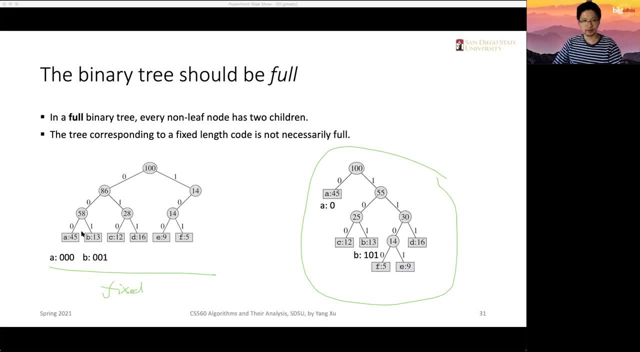 most efficient way of encoding, right? so if it's a fixed code, then you will see that the node for this one, for this 14 node, there's no left, uh, no right. uh, uh, branch, okay. so this is something that you can immediately test and you can immediately test. and you can immediately test and you can. 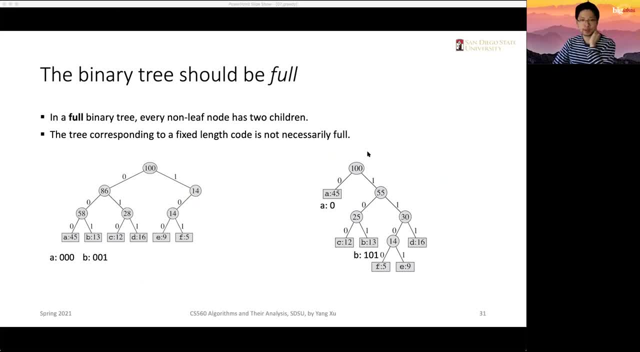 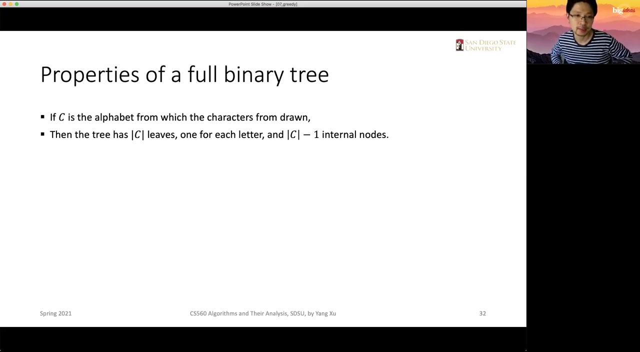 tell from the shape of the tree that you have grown. okay, so what we essentially want is something like this: a complete tree that each internal node have both children. okay, all right, some further properties for a full binary tree. and let's use this capital, c, uh, to indicate the uh alphabets or the vocabulary like c basically is a set of. 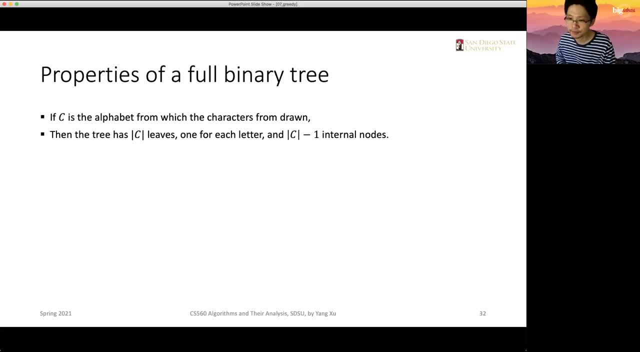 all distinct uh characters used? um, that's a good question. i see a. i see a question that's uh. um, in this i'm gonna resend it. so it is a how ask to code work? uh, i don't know i need to. i need to look into that. um, not sure, though my feeling is. 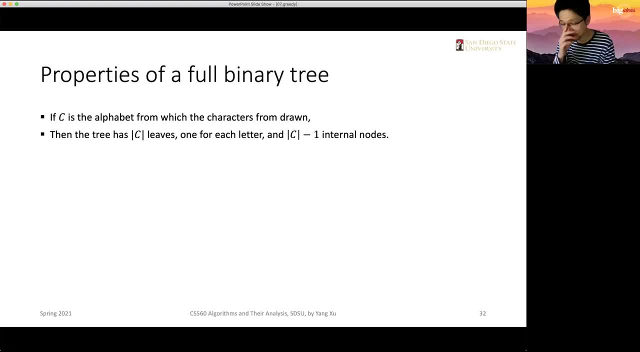 that it is not okay. so, uh, because at least, uh, uh, the ask code, ask to code for the letters, should have, um, they are just integers, integer numbers, right, right, they are not, um, uh, binary encodings. yeah, i haven't thought about that, yeah, but uh, it's interesting to look into. so, um, back to the binary tree here, so we use the capital c. 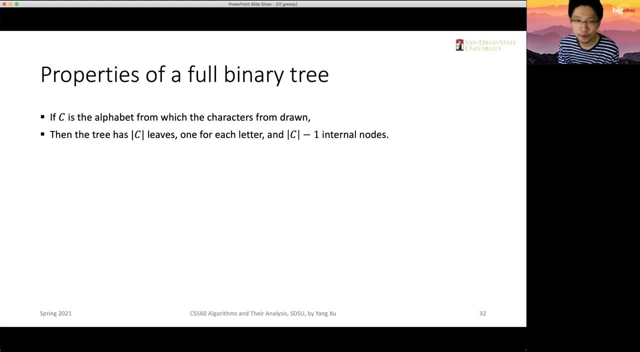 to indicate the complete set of all characters. okay, then the tree: we use the size, so this size of the set actually is the number of, uh, leaf, nodes or leaves in the tree. okay, so one leaf is for each letter, okay, and there are cestres, another xys, right? 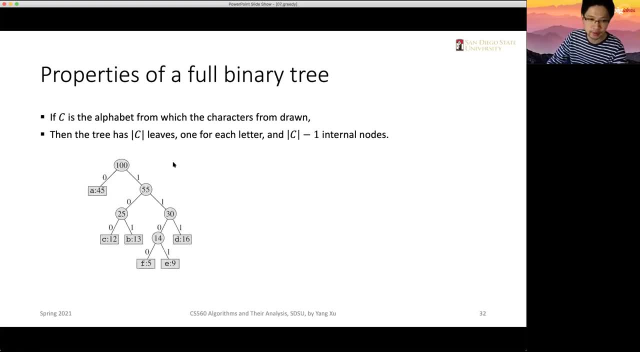 minus one the size of c, minus one internal nodes. okay, so that is something uh, you can examine quickly on to from this, uh, um, the example trees: we have one, two, three, four, five, six, six leaf nodes, uh, for six letters, and the internal nodes are those circles. right, we have one, two, three, four. 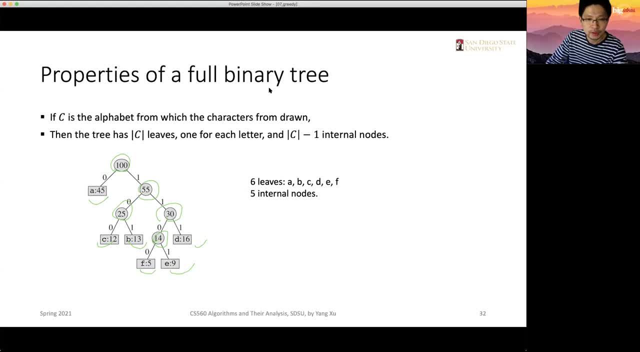 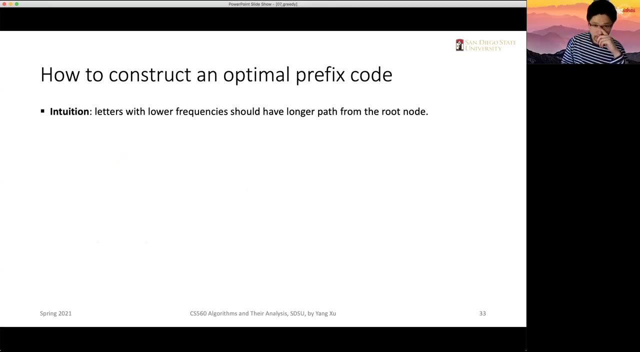 five, five internal nodes. okay, oh yeah. so now the question is that how we can actually construct a optimal prefix code. okay, we are, we actually already know the intuition right, because we want to um um for those frequencies that have, uh, lower, for those letters that have free, uh lower frequencies. 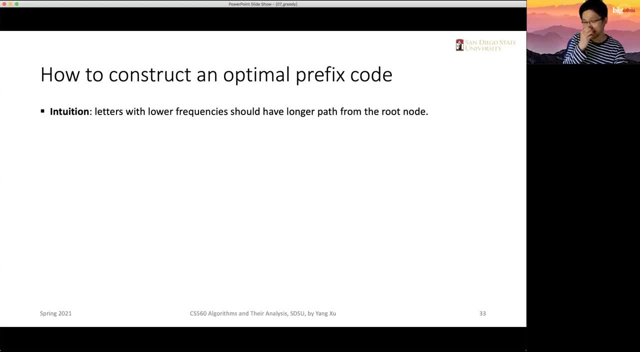 they are like rare letters that don't appear a lot in uh in our data. then it's okay that they have longer paths from the root node, right, which means they have longer codes. yeah, because they're rarely used, so it's okay we assign some longer codes. that's a rational choice, right, and for those. 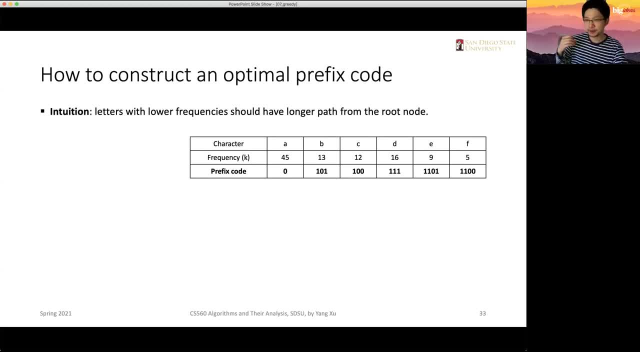 that are on the other, on the other, obviously, like uh for the for the more frequent letters. of course we want to uh save space, right, because they're used so often. so it makes sense to just use one or two or even shorter. just use as few as uh codes as possible for those frequent letters. okay, so, uh, it's basically the. 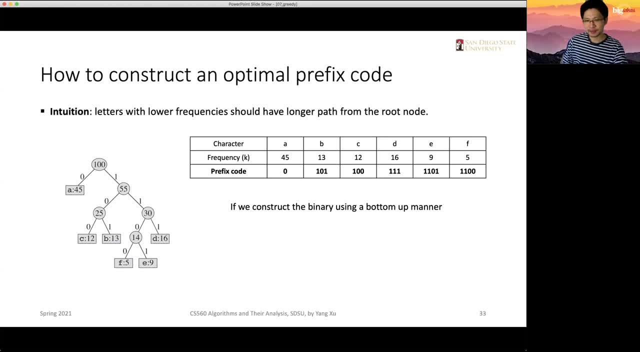 following this intuition, we can like construct the binary tree using a bottom-up matter. okay, like we can start from the least frequent letters and then we put them into the bottom of the tree and then grow this tree from the bottom-up style using a bottom-up style. okay, so we should uh select. 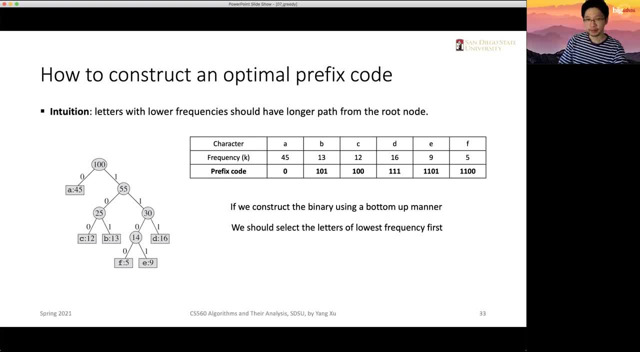 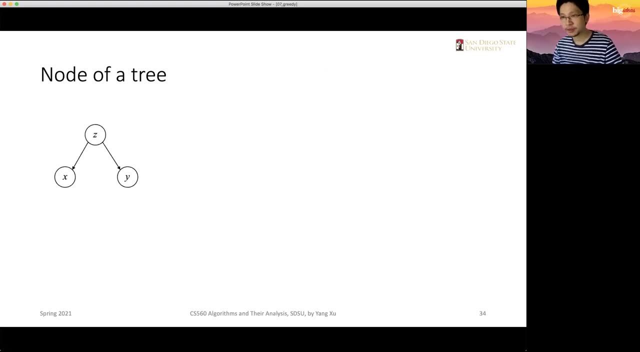 those letters that are least uh frequency in our vocabulary. okay, in this case it's the letter f and e. right, one has five and one has nine uh frequencies. okay, so, uh, again, let's uh get some preparation by looking at how trees are uh uh constructed. basically, uh, we need to have a node, right, the node here in the middle, it's the so-called parent. 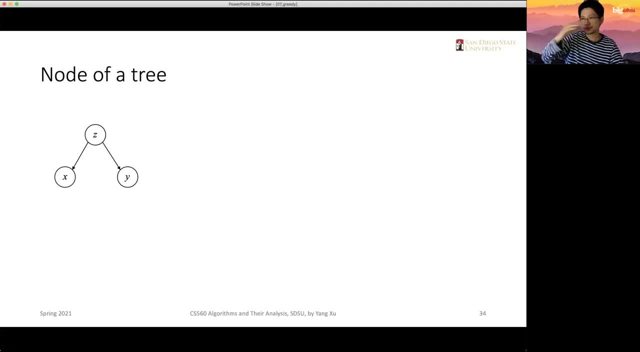 node. it's at upper level and it has two branches, one pointing to the left child and the other point to the right child, right, so we in in a tree node, we can, uh, using this pseudocode convention, we can use the z dot left to indicate that it's the, the, the left child for the parent node, z okay and the zd. 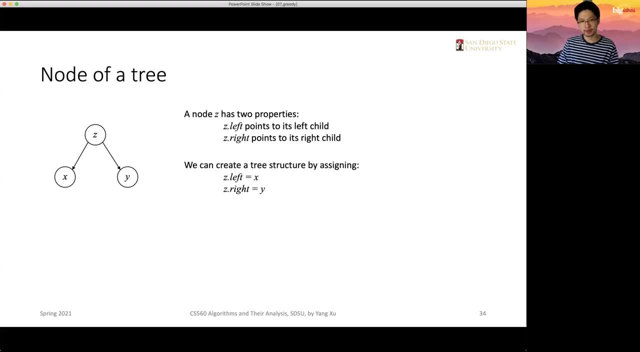 dot right points to the right child of the parents. okay, so we can create a tree, basically by assigning some other letters or other nodes to the left? uh pointer over of a parent node right. so like we can construct the parent node z? uh by assigning the node x to the left pointer of z right. use this: 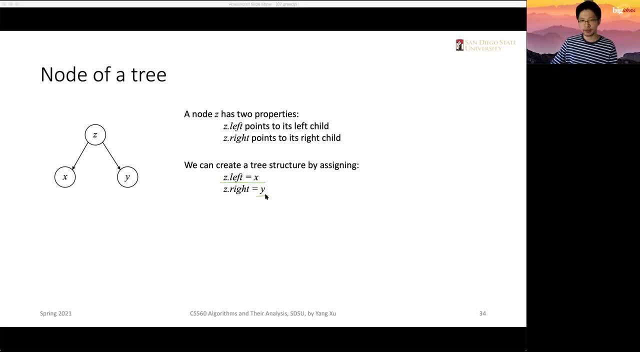 assignment statement. okay, and we let y the node to be to assign to the the right pointer of the parent node. all right, so, and we can also easily uh check whether a node is a leaf node or not. so we basically look at whether the left child and the right child pointers they are nouns. 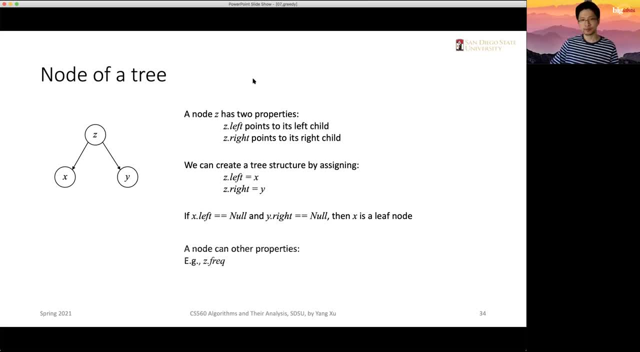 okay, if they aren't all nouns, then it's a, it's a leaf node, okay. and in our particular example here we, in order to visualize the whole process, we will also attach the frequencies for a letter to each node. okay, so we can access the frequency for each node. 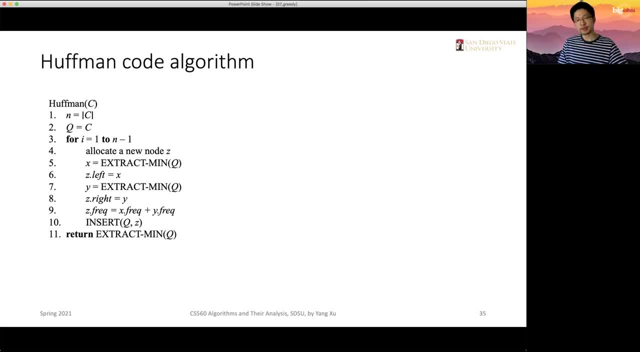 quite easily. all right, we have everything ready now and let's look at the code for halfman coding: uh. halfman code algorithm. so it's uh. uh takes inputs the, the vocabulary, or the, the alphabet, c, it, which is a, which is a set of n characters. okay, uh indicates the. 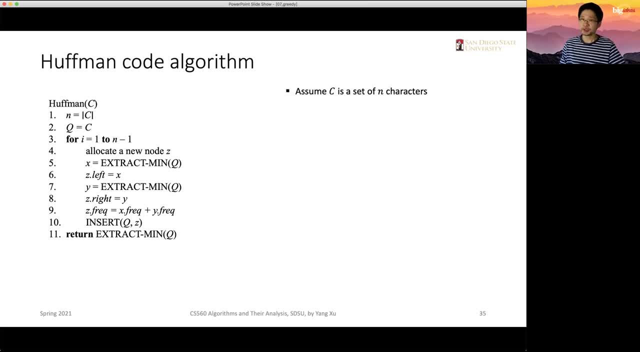 n unique characters that have appeared in our data. okay, and for each character we will have a frequency attribute by c dot freak. okay, so the first line is to count the size of the c, like how many letters we have, and the second is to use the song. you only have one for each column, which is a. 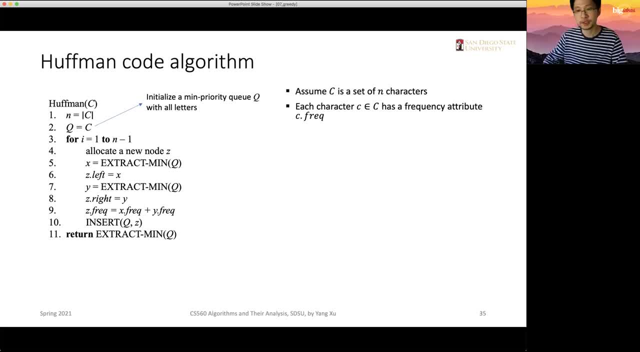 percent of the number and, uh, so we, yummy, will have less than the number filled here. so that, actually. and the second is to use a minimal priority queue. okay, So this minimal priority queue, it's like a queue data structure that's, in which all the elements 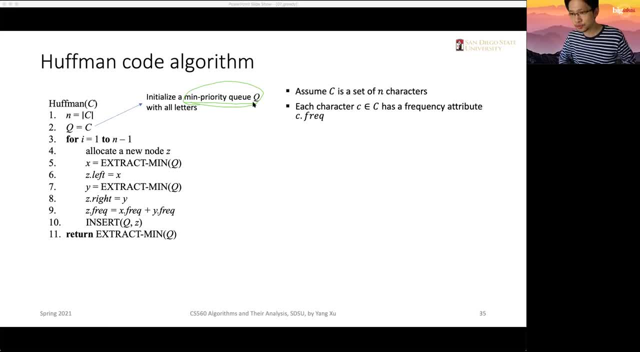 is assigned with a score- okay, And this score indicates a priority of the queue, which determines whether when that element is gonna be dequeued, So the elements that has the highest priority will be the first one being dequeued. So that is basically how a priority queue means, okay. 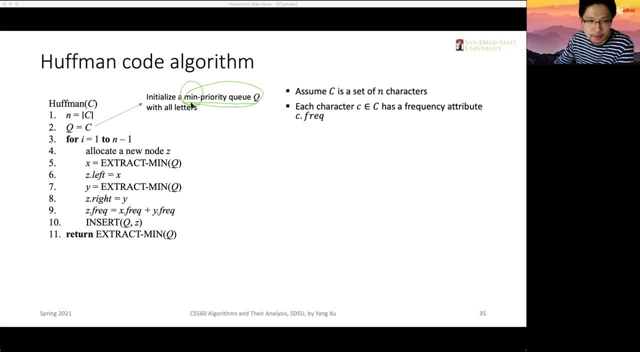 So what about this minimal priority means? So this minimal priority means that the elements that has the minimum score in that queue will have the highest priority. okay, So it sounds like two concepts. it's the priority, it's the score, it's the score right. 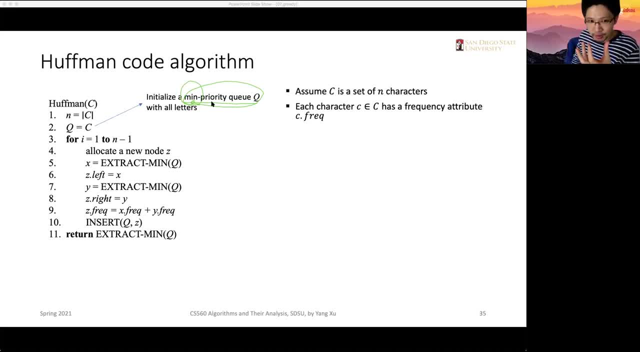 So we can basically say that the smallest elements in that queue will get dequeued first. okay, Now, regardless of the order of when that queue entered, the one that elements entered the queue- okay, All right. So this data structure is something we're gonna use. 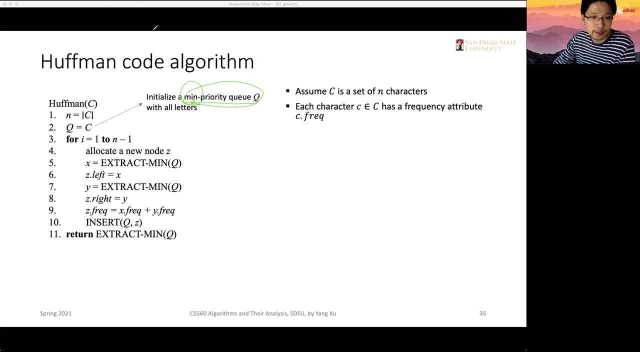 for store for all the letters. So we're gonna initialize the minimal priority queue with all the distinct letters we have, okay, Then we will have a for loop, okay. So that's the minimum priority queues. okay, So the queues will support the operation called. 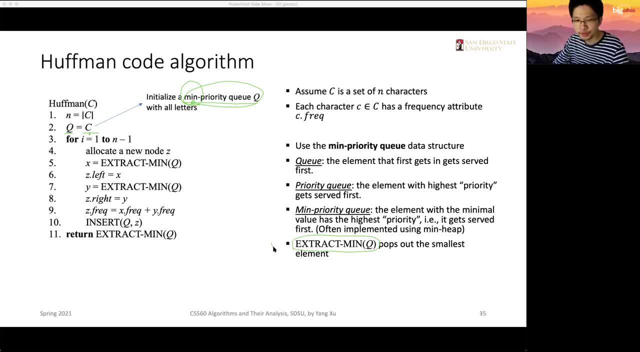 extractMinimalQueue. okay, So this extractMinimalQueue is something, is a process or procedure that's gonna let the smallest elements in the queue pops out. Okay, So this is a key operation that we will use. okay, And also there is another operation. 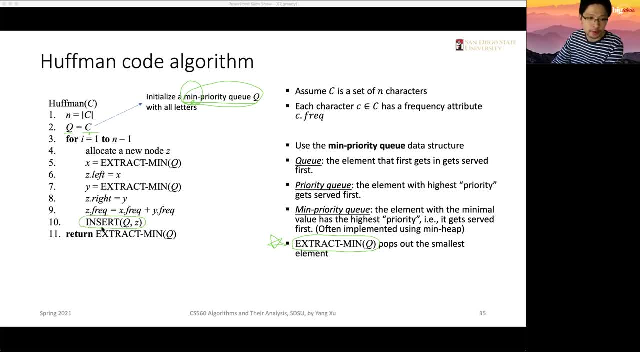 that is for the minimal priority queue, which is insert. Okay, So this insert is just to insert some elements into the queue, Okay. So let's see the body of the for loop. okay, And it's a quite straightforward code. The first, the line four, is to allocate some new node. okay, 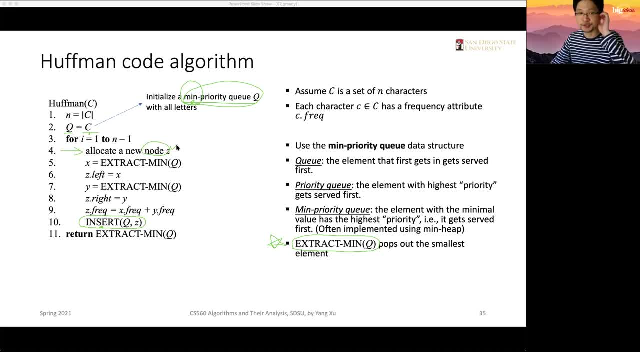 So this new node is something we created at the beginning of each step. okay, And how do we create that Z? Is that we need to first extract a minimal elements from the queue. So the X is the one that we extracted from the queue. okay, 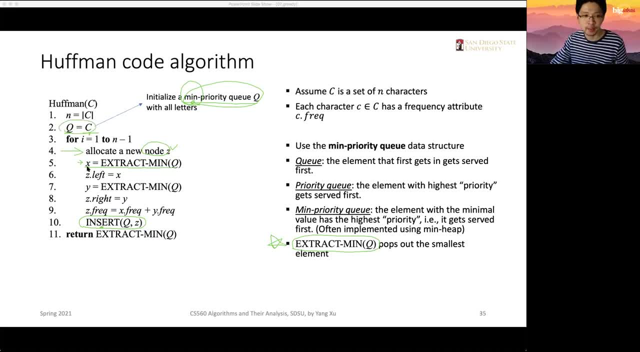 So at the beginning the queue is full of letters, right, So we can extract one element out. So what we do with X is that we assign X to be the left child of Z. So it basically looks like this: We will put a Z here. 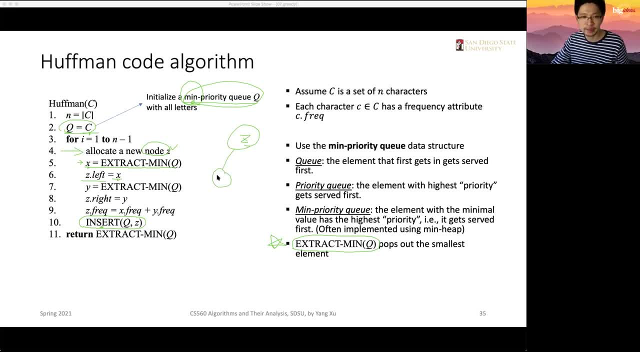 Z is the empty node, okay, At the beginning. And then we will assign the X to the left of Z, And then we extract a second elements from the queue, okay, So, other than X, because X is already popped out, then the y will be the next smallest element in the minimal priority cube. So y will be. 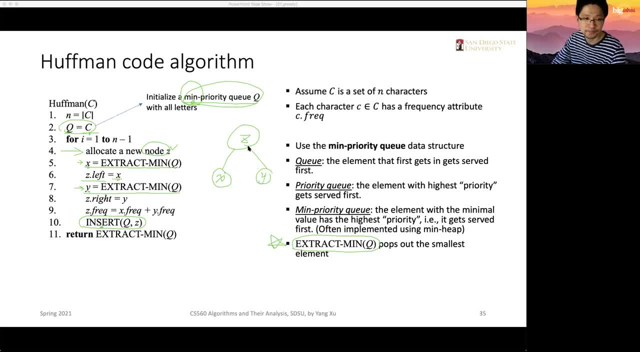 extracted and it will then be the right node of the z. Okay, so the line nine is that we compute the summation of the x node and the y node and we put the summation to the frequency attributes of the z node. The z is the new node that has been constructed. 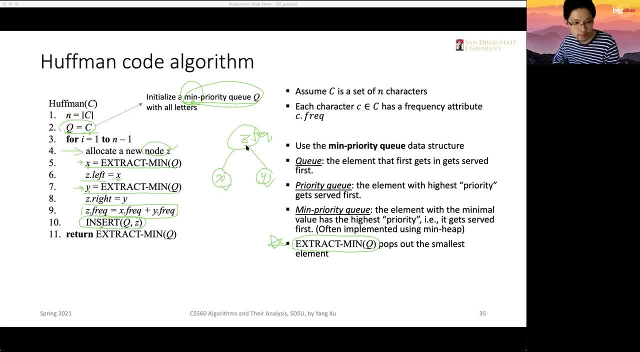 Okay, and we need to put the z, the new node z, back to the cube. Okay, but it's not put x and y back. x and y are already popped out, but we'll put the z back, So z is a new object in the memory. 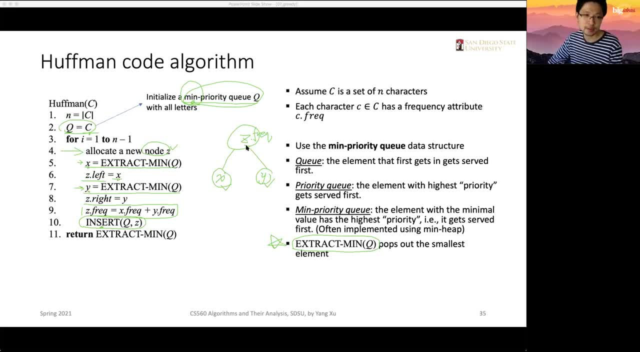 space. It's a new node. Okay, so that means in each iteration of the for loop, like we extracted two elements out and we insert one element back, So the size of the cube actually decreases by one. Okay, so this is a decremental algorithm. So whenever each iteration will, 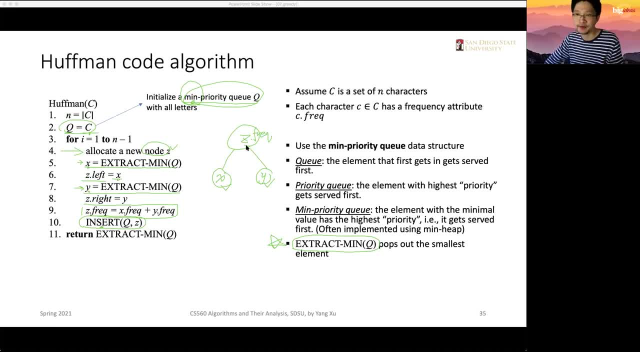 decrease the size by one. So eventually we're going to have just one element in that minimal priority cube, right? So we let this for loop iterate from one to n minus one, right. So when this for loop ends, there's only one element left in the minimal priority cube. So 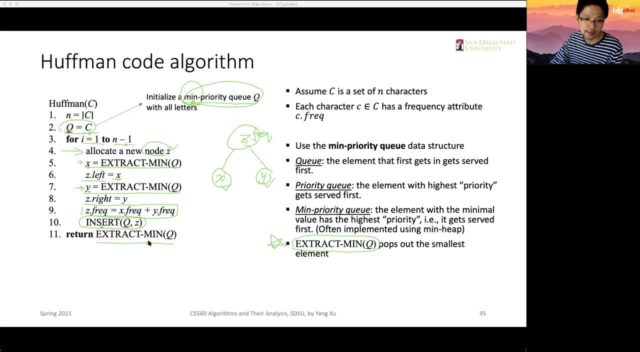 that's why, eventually, we're going to extract that last element from the cube and return it. Okay, so the returned node is the root node. that points to all the elements that contain a. that contains a complete Huffman tree. Okay, All right, so let's use an example. 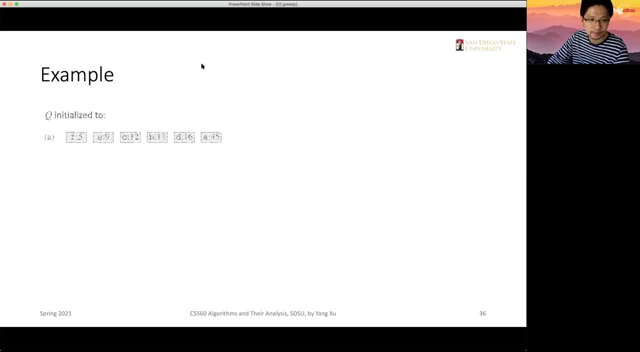 Since we have the general CT relation of two units and any of the elements that I have already eyes. Okay, let's use an example of first 괜찮아 to the first ta and put one of the elements to the secondки. 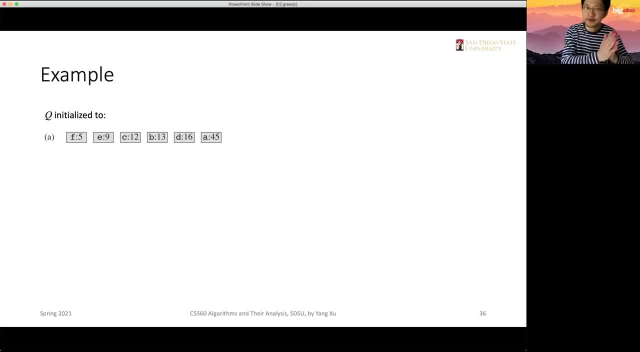 Another example is Tla E And let's take look at an example where readiness of�� is set to zero, of Tfa like this and a limit versch to 0.. And that is the quoting and circle in the table. in the table. 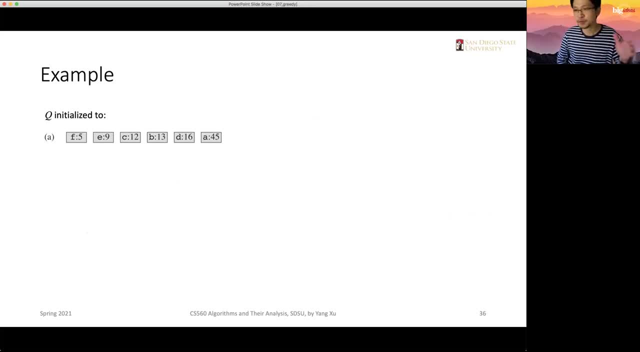 are ordered by the frequencies, So the leftmost one has the highest priority. It will be the one first being extracted. So extract the minimum. prior to Q will pops out the note for F, right Letter F, And according to the algorithm, 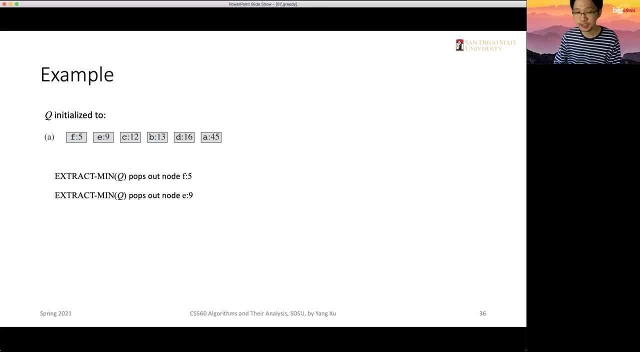 we need to extract two notes, and the next one will be the letter E, right, Because it has nine as the frequency. So now we're gonna make a new note Z, right, And the F will be the left child and the E will be the right child. okay, 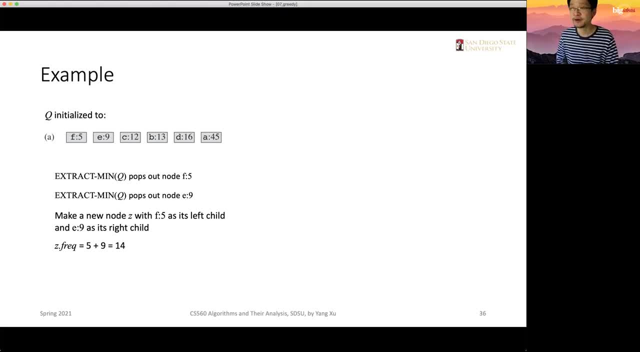 So the frequency attributes for Z would be five plus nine, which is 14,. okay, Now we have this new structure constructed, So we all have a Z, new note Z, and then this Z will be inserted back right. New note Z will be back to the Q. okay, 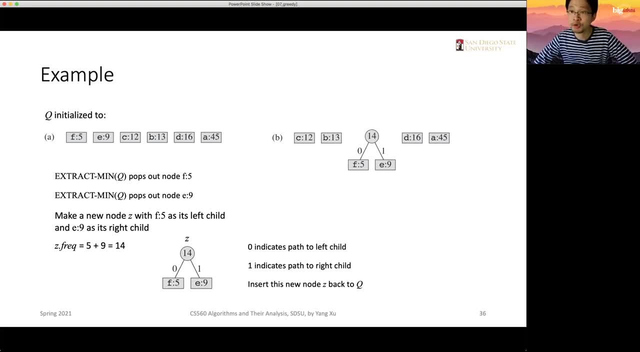 And by inserting it to the Q, which means it will be appeared. it will appear at the correct position because it's a minimum priority Q That it has. the note being inserted has the frequency 14, and which means it will appear at this position. 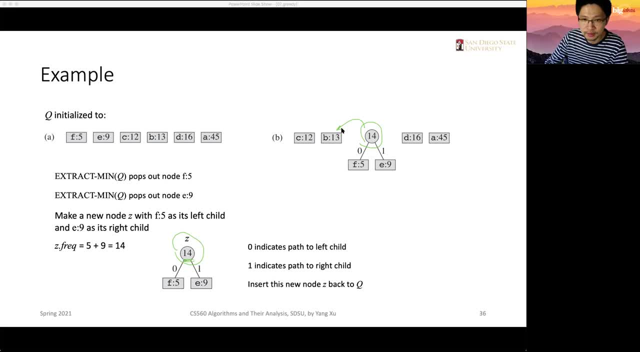 because it has lower priority than the B and it has higher priority than the letter D. right, Because the frequency is in middle. okay, So that is how the they find, basically how the minimal priority Q maintain the sequences for all the nodes in it, right? 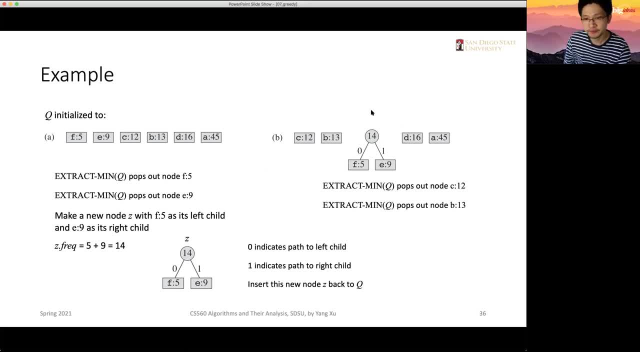 And we will let these procedure continues, okay, And then we will further in this second iteration, we will extract the letters right And after they are extracted they will construct a new note and this new note will be inserted And this CNB: the frequencies add up together to 25.. 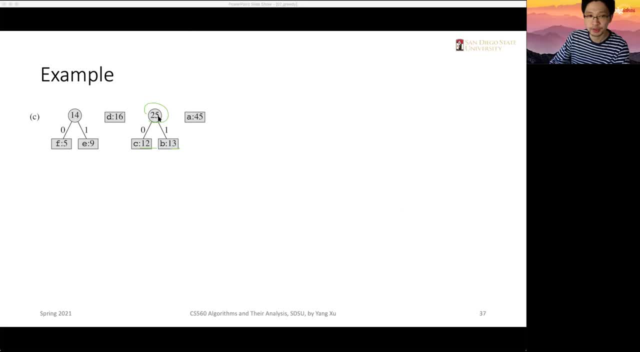 So this new node will be inserted to this position because it's higher than 16 and lower than 45, right. The next iteration is going to be a little bit different because the extracted node would be the node that we created in the first iteration, right. 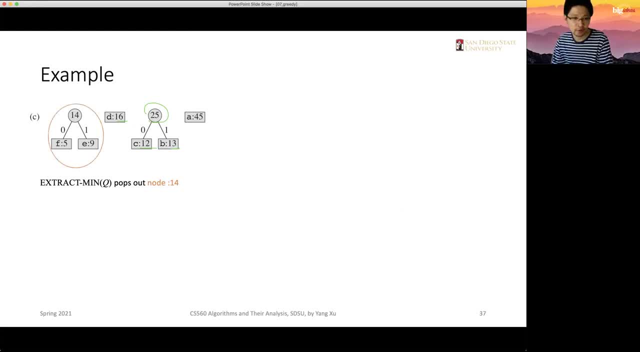 It is the node Z, right? So this new node will be extracted altogether as a complete unit. as a whole unit, okay, And the next one would be the letter D. all right, So now let's merge them into a new node. 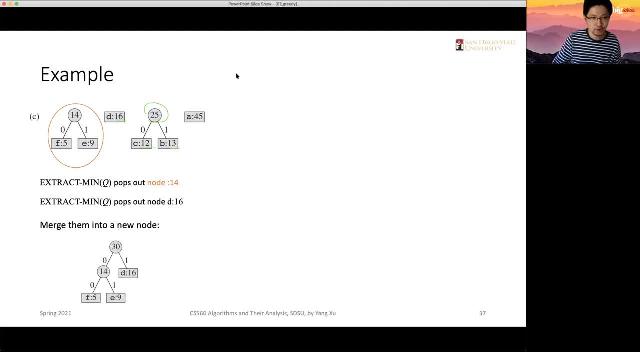 We just follow the same principle. right In this new node, the left child would be these parts, which is exactly node that we extracted. okay, Because the frequency frequency is 14, which is lower than the frequency 16 here, right? 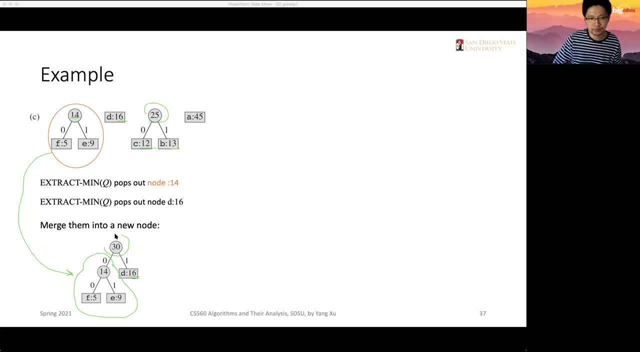 So the new node created is actually this root node that has a summation between 14 and the 16, which is 30, right? So this is how we construct a node with two nodes, right? The first node is itself a composites of other nodes. okay, 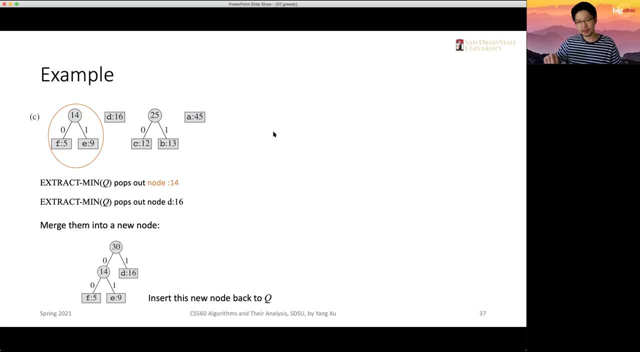 So, yeah, we have a very big node now, and that big node with 30 as the roots node elements will be inserted back as well, okay, So this 30 will be inserted back and now it's in the correct position right after the node 25, okay. 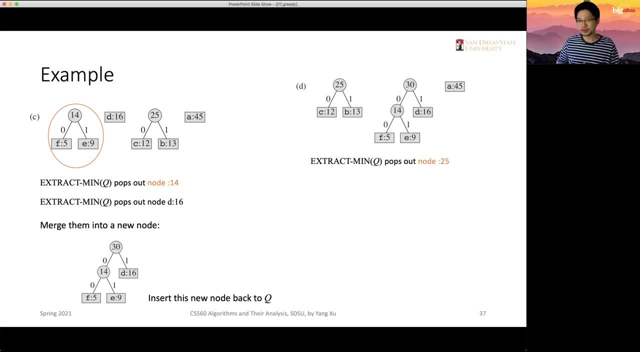 All right, so we will continue this until our minimal priority queue is empty, right? So the next one being extracted, the next two being extracted, will be these two nodes, and we're gonna compare their node, their root values, right? 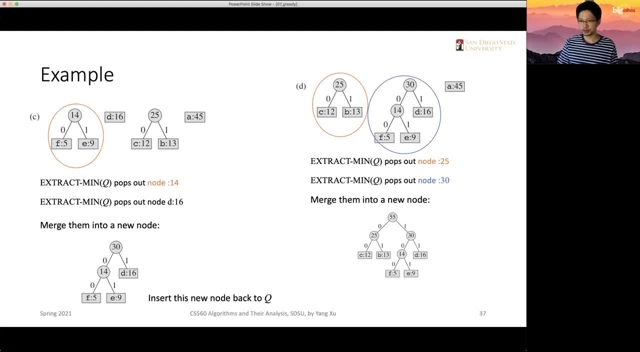 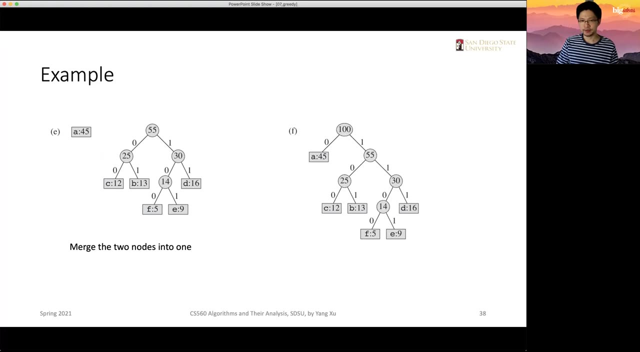 And we compare an even higher, even larger nodes, which gives a which has 55 as the root node- okay, And this node is again inserted back. okay, Now we have the last two elements, so we will extract them all and construct a final node which has 100 as the root node. 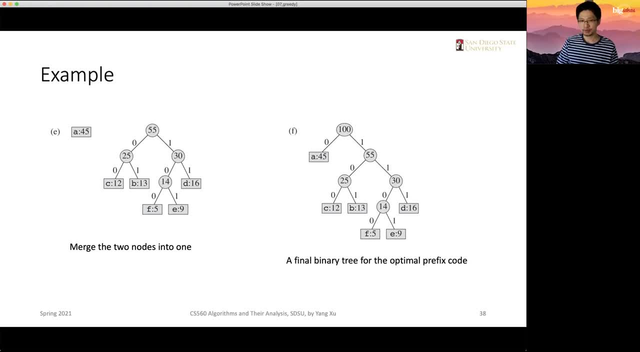 which is the root node value, And this one will be inserted back into the minimal priority queue And at this point our for loop is also done. right, Our for loop is done and this one will be extracted, will be returned. okay. 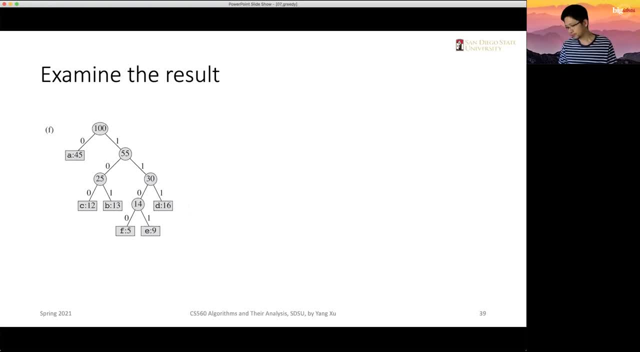 And this is exactly what we need in order to construct a Huffman code tree out of the frequency table. okay, We will. simply, we will need to utilize the data structure called the minimal priority queue. okay, And if we examine all the passes from the leaf nodes to the root node, 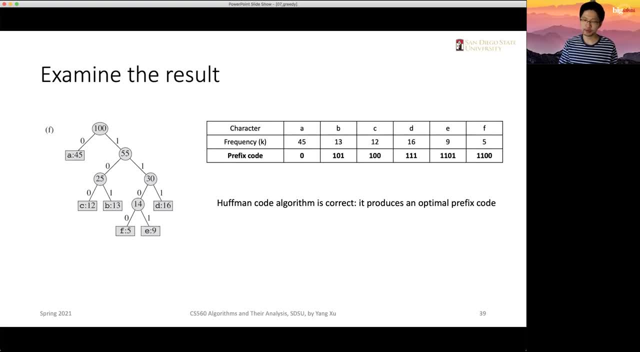 we will find that it is actually correct. It produces an optimal prefix code. okay, So actually the correctness. how do we prove the correctness of Huffman code? algorithm is pretty complex and it's not required, but if you are interested, you can read the proof yourself from the textbook. okay, 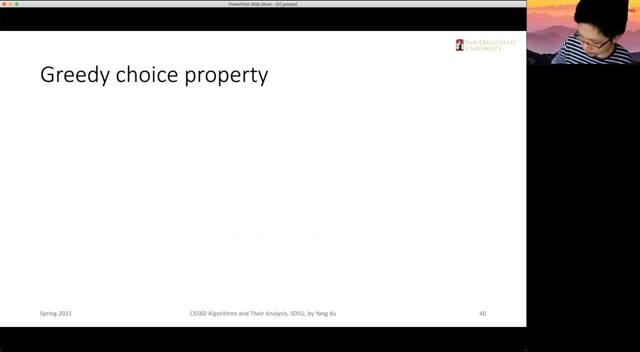 So let's look at this Huffman code algorithm and we it belongs to. we can categorize it as a greedy algorithm because it's making greedy choices in each step, right? So the core concepts that is of our interest about some encoding is that we want to minimize 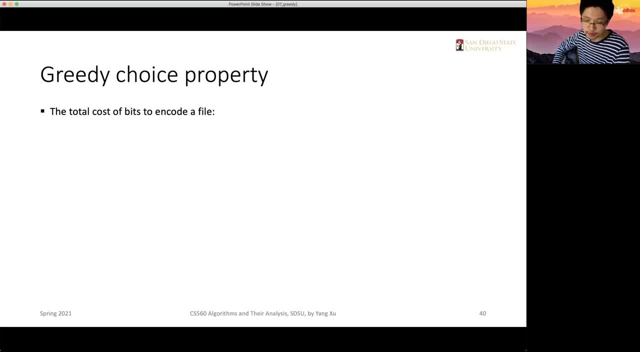 the total cost right To encode the file. We want to use as fewer bits as possible. That is our goal, right. So the total cost in this particular example would be the summation of a couple of a bunch of products, And the product is between the frequency. 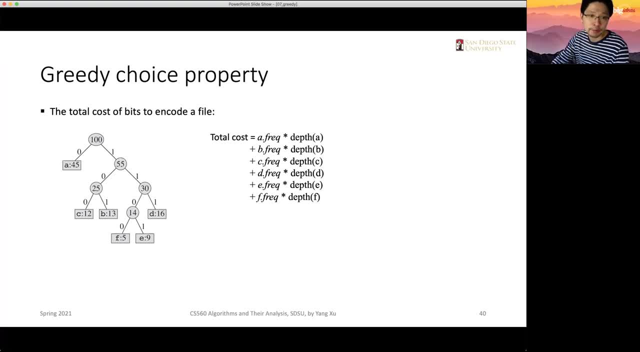 and the depths of a node, right? You see, when we want to compute the total cost, we need to look at: okay, A is here, It has frequency as 45,000.. We need to use that to times the depths of A. 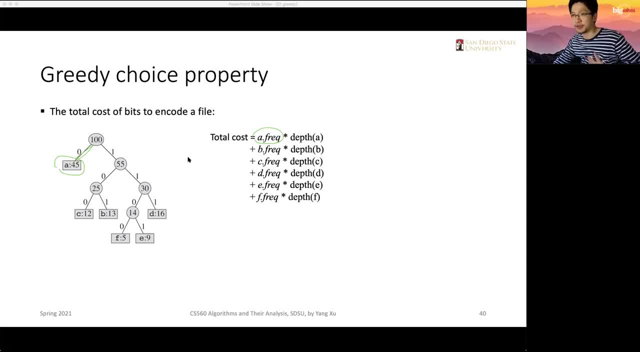 which is the, which is also the length of the node right, Which is also the length of the node right, Which is also the length of the node right Of the optimal of the encoder of the Huffman code. so it will be the depth of A. 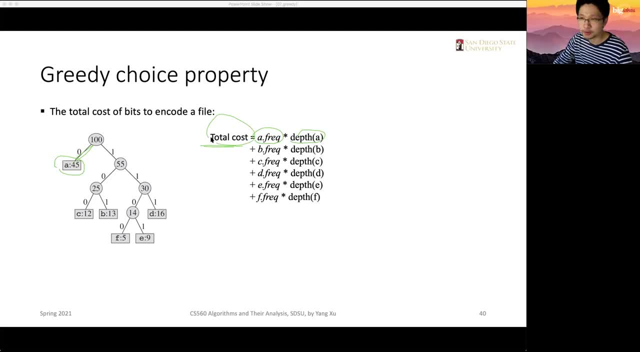 So these total costs would be our goal to minimize right. So if we represent it with the cost function, it'll be like this right It will be like to: we want to enumerate over all possible characters in the data And then we'll use its frequency times. 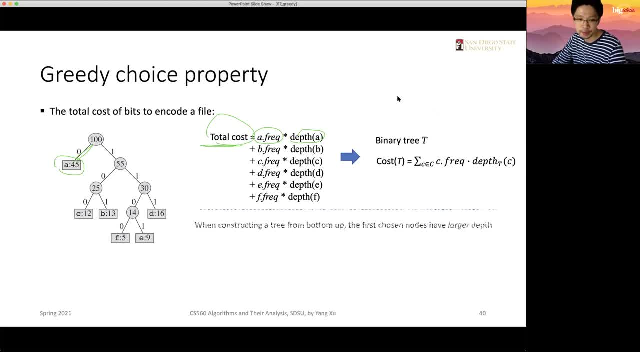 the depths of that letter. Let us see in the tree. okay, So when we construct a tree, use this bottom-up matter. we will first the first chosen nodes right. The early picked nodes will have a larger depth, okay. 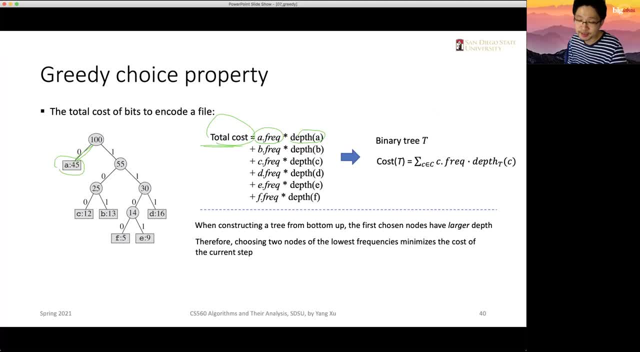 So, therefore, it makes sense that the greedy choice is to choose the two nodes that are lowest frequencies, that are the lowest that has the least frequencies to, in order to minimize the cost of the current step. okay, So you see, the key is that when we choose, 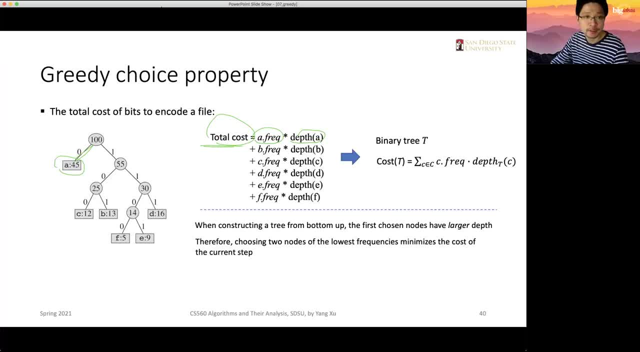 the lowest frequencies. when we choose the two nodes of the lowest frequencies, we are not sure whether this gonna minimize the goal, the global goal, Whether we are not, whether we are gonna have a final minimize cost. that is something we are not sure. 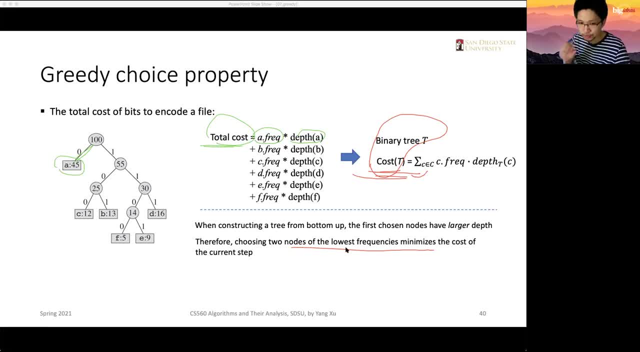 We just know that by choosing the two minimum frequency nodes will minimize the cost of the current step. okay, That makes our the current choices make sense. right, We want to choose those elements that has fewer frequencies Because they are at the bottom. 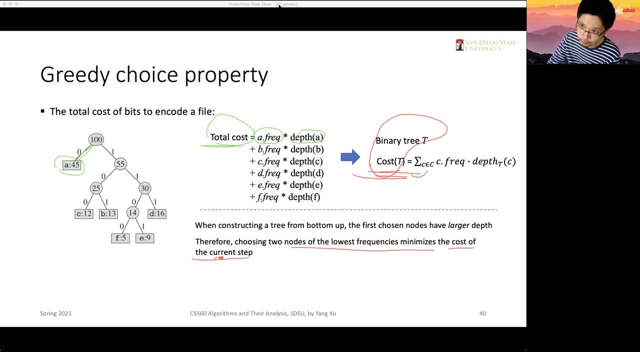 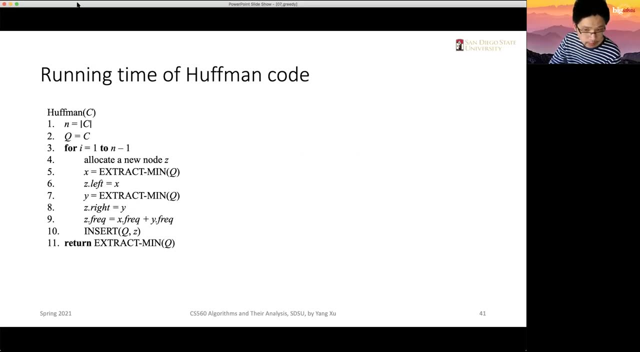 near the bottom of the tree, okay, But we don't know whether this is gonna be a globally optimal choice. So that's where the greedy choice property is from. All right, So let's look at again, look at the running time. 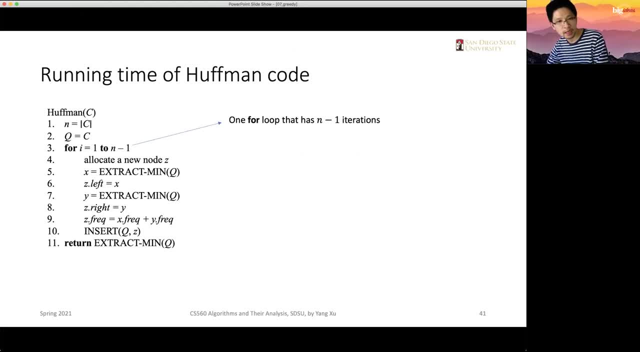 of this Huffman-Coles algorithm. It's a. it's structure wise, it's pretty simple algorithm because it has just a one for loop and the iteration is determined right. It's like n minus one iterations, okay. So the thing is that we have some. 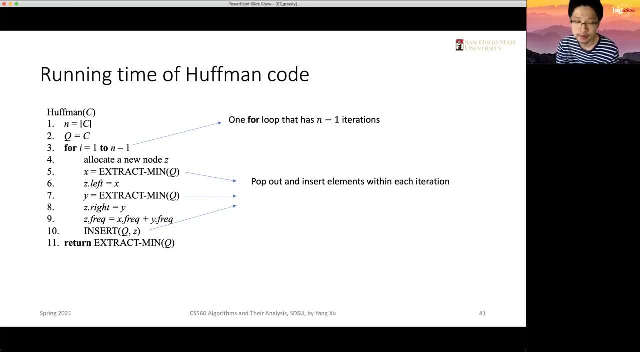 calls of these extract minimal elements of the queue. okay, So it depends on the data structure, the minimal priority queue data structure. right, We need to look at how fast the data structure is in supporting the pop outs and inserting procedures. basic operations. 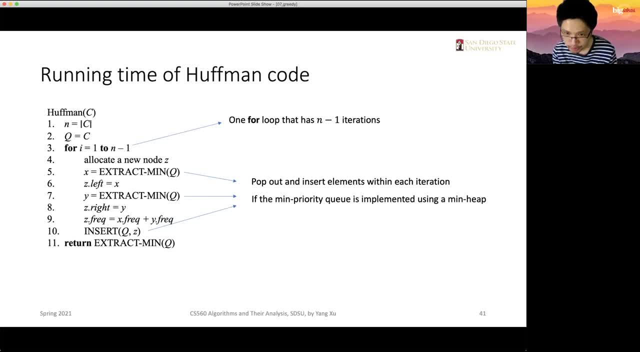 right. So the minimum priority queue is actually- we actually have mentioned that a bit- when we introduced the heap sort, when we use the max heap, right? So we? I remember there's a slide showing that, saying that the minimal heap can be used to implement the minimal priority queue. 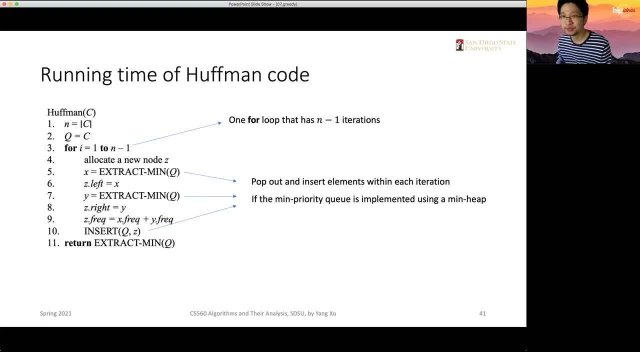 okay, So a little bit review here. a heap is like a tree structure, right? So then the max heap that we use for a heap sort is that the parents node always have bigger values than its children node, So the minimum heap is the opposite, which is that the small 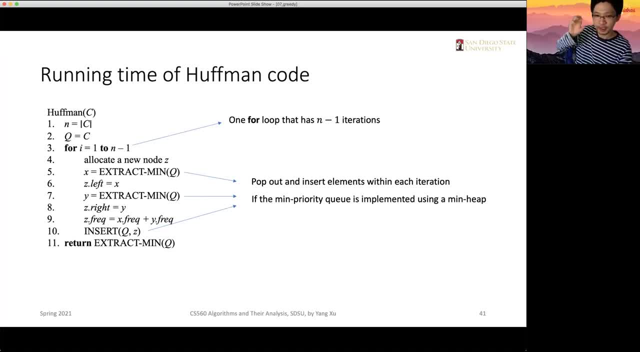 the, the top elements, or the parents elements. the parents node has smaller values than the children nodes. okay, That's for the minimal heap, okay, So if we use the minimal heap to implement this minimal priority queue, then we're going to have a logarithm. 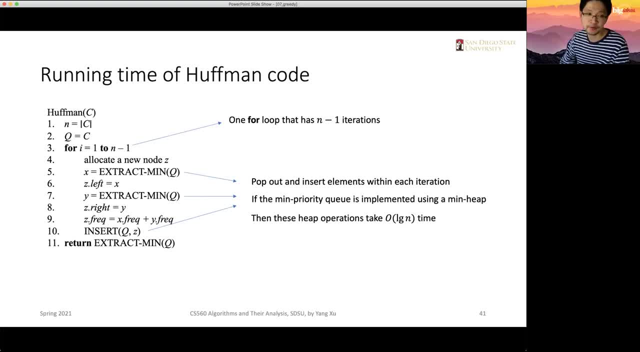 of n running time for these heap operations, for this extract, mean and insert elements operations. okay, So it's just a little bit similar to the max heapify procedure. It's like whenever we change the positions of the elements in it of its like, we extract the one element out. we need to like use max heapify or minimal heapify. 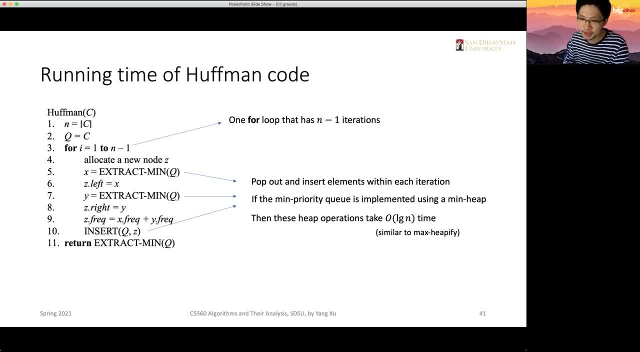 in order to maintain the, the max heap or minimal heap, the mean heap properties. okay, So it's a more complex даy好吧, in term of the shortest file type, kind of associated with a command response. So before we Посol Song hearing the people come and go, So let me give a little bit, pull up a comment. 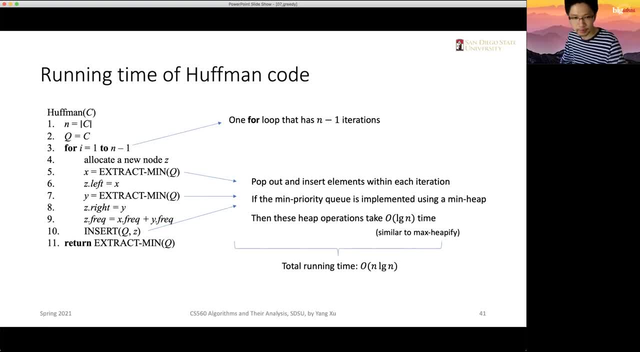 I just want to comment about the other stuff here. So the last slide again goes a bit further. So있im this part you can find the best tasting voice yourself. So altogether we have logarithm of n basic operations within the body of a for loop. 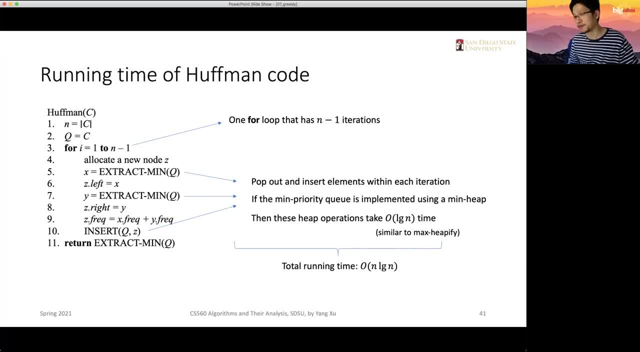 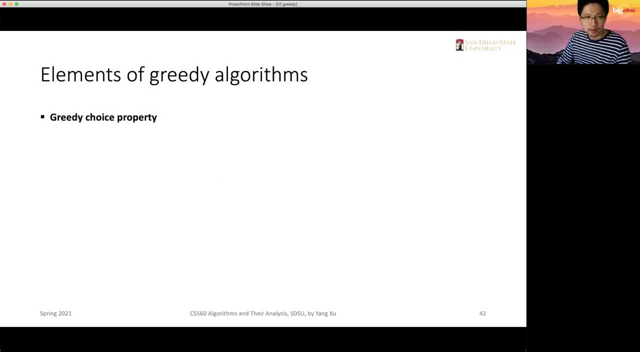 So altogether it's going to be big O of n times, logarithm of n running time, efficiency, All right, so let's finally review the Guidi algorithms a little bit. okay to look at the elements of the Guidi algorithms so far. So by Guidi choice we mean that. 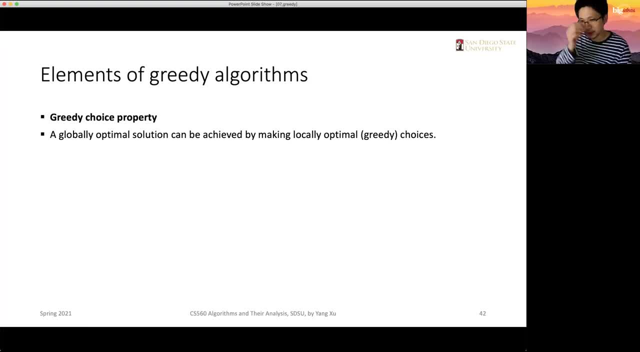 the globally optimal solution can be achieved by making locally optimal. Okay, so this locally optimal choice is the so-called the Guidi choices. Okay, so we make the choice that it looks best in the current problem, but we lack the information. There's no information telling us that these results, whether these results are going to be, 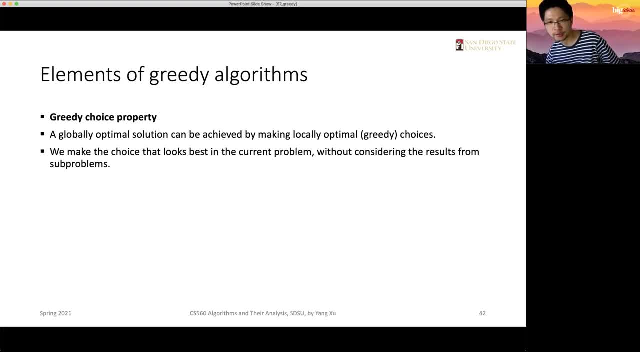 lead to the globally optimal ones. So we don't consider the results from all the sub-problems And the GUI. algorithms usually also represent some optimal substructure, also can reflect some optimal substructure which is similar to the dynamic programming algorithm. That's the solution. the optimal solution to the original problem contains optimal solutions to. 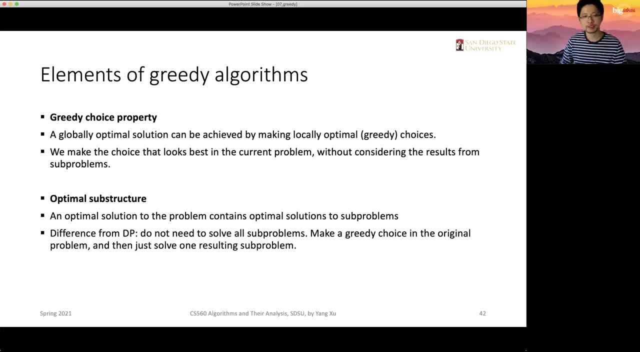 the sub-problems. But the thing with the difference with DP is that we actually do not need to solve all the sub-problems for a GUI algorithm problem, because these particular type of problems make sure that making a GUID choice in one original problem is enough. We don't need to. 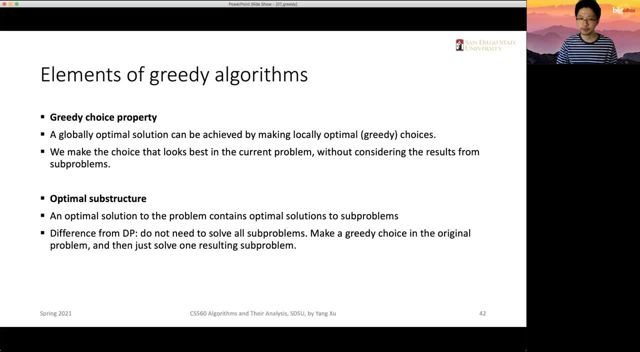 compare over the solutions from all the sub-problems. we just solve one resulting sub-problem using some simple heuristics. So that is the connection between GUI algorithms and a dynamic programming algorithm programming. All right, Let's look at the last example for 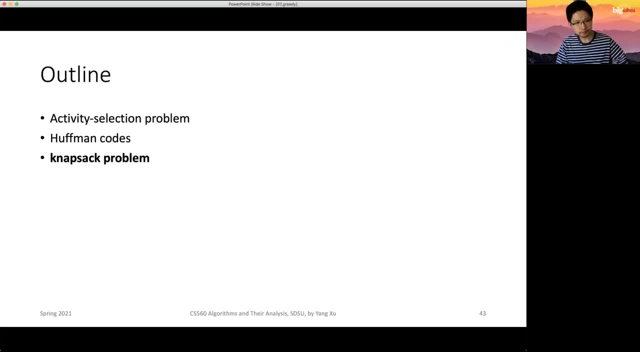 greedy algorithms. Okay so it's actually pretty. So we will draw a connection, we'll draw a comparison with dynamic programming in this for this problem. Okay, so there's actually two types of knapsack problems: The one, the first one. 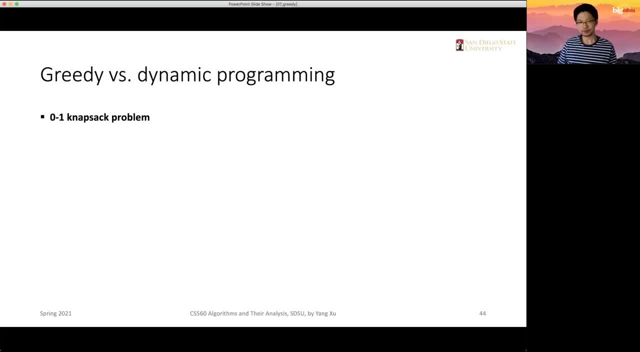 is called zero or one. Okay, so it's also called discrete knapsack problem, And it's quite easy to understand actually. So it's like a thief. That's how the original problem is defined. It's like a thief robber in a store and he finds that there. 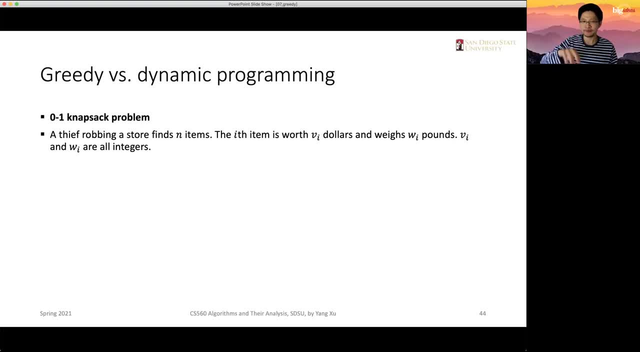 are multiple items to take. okay, say, assuming we have n items. okay, and he knows the value for each item as well and the weights as well, Okay. So, for example, the ice item has the value of vi and is has the weights wi. Okay, And and. 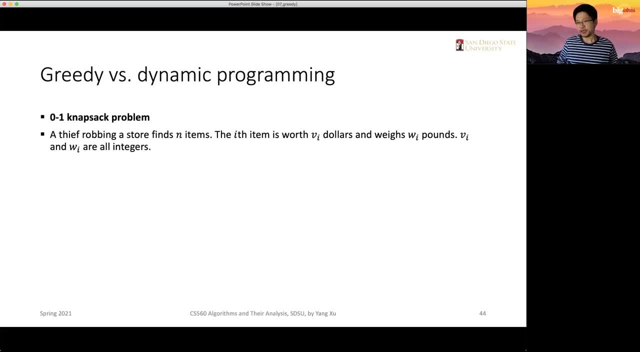 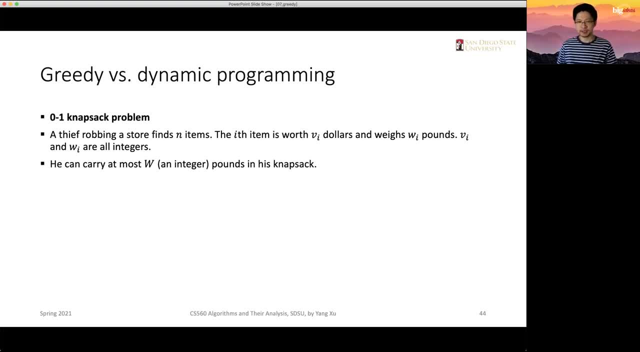 has a limited capacity in his knapsack. Okay, so he can carry at most W pounds. So, at most the W pounds, and the goal is that to, to, to optimize, optimize the values. okay so he wants to take as many objects. 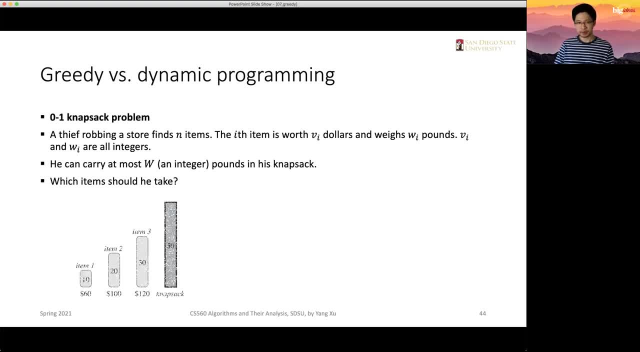 and then many items that are as valuable as possible. Okay, So in this simple example here, if he has three items to choose from, right, the first one is worth $60. And it's very light right, it's just 10 pound weight. And the second item has $100 value. 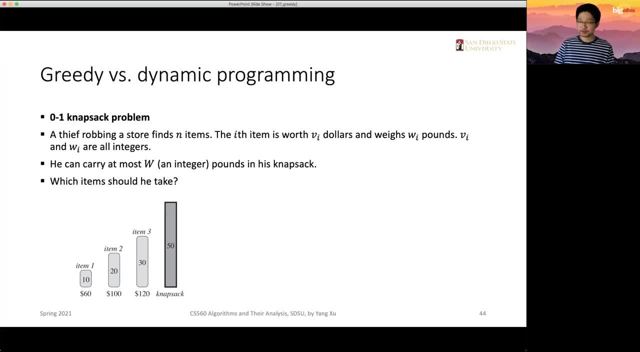 but it's heavier. it has 20 pounds. The third one is the most valuable One, but it has it also the heaviest: it has 30, right, 30- pounds. So, given a capacity that is like 50 pounds in total. 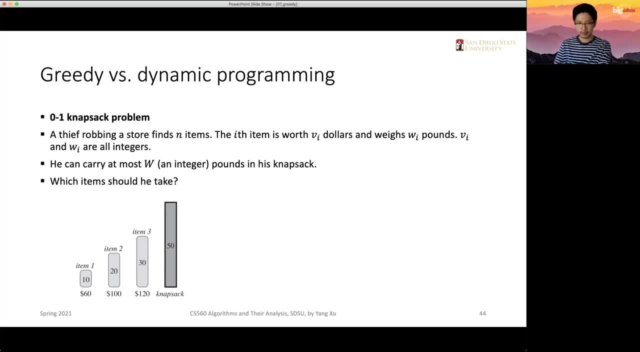 right he can carry out, can carry 50 pounds at most sent. So what would be the best choice? So I think in this example it would be easy to enumerate all possible combinations, right, So like if he takes item one and two, it'll be like 60 plus 100, which. 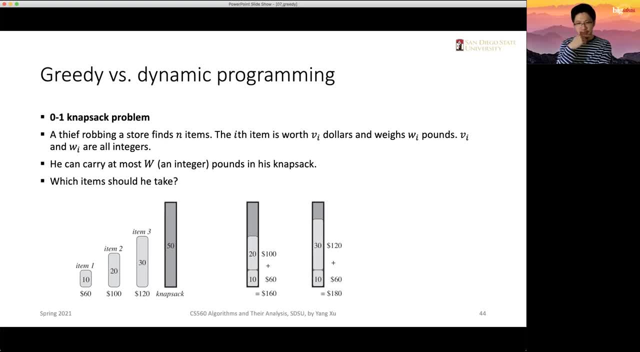 is 160,, right, If he takes 10 plus 30, if he takes the item at a one item three, right, it's still within the capacity, right? so it'll be 180.. And, of course, if you use the most of, 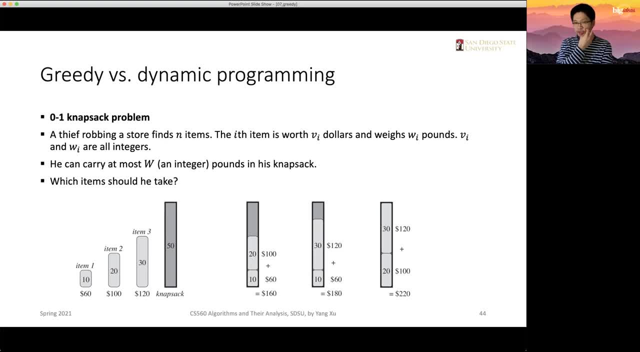 these knapsack, it will be like 100 plus the product, which is like 220, which optimizes the his like revenue or his outcome, right, So that's, that's a pretty obvious solution in this simple case. Okay, But if we got, 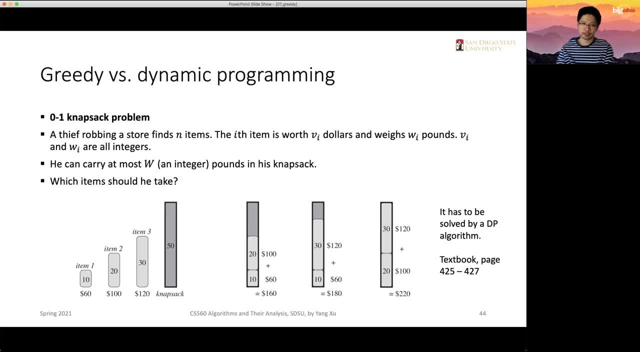 a general solution. if we want to get a general solution out of some more problems and we want to solve that problem in an efficient way, then this problem is not that easy. Okay, so it has to be solved by a dynamic programming algorithm. Okay, And I'm not. 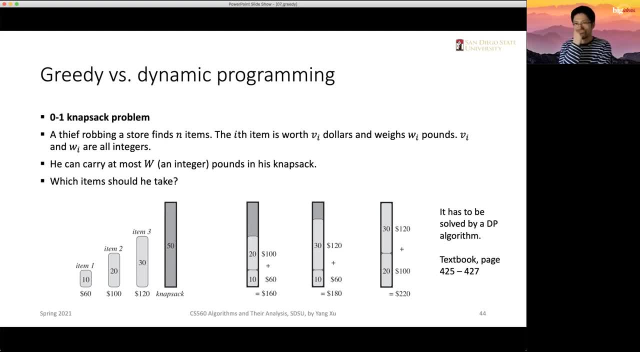 going to show the solutions for a complete solution here, but you can actually find it from the textbook in those pages. Okay, So well, this is just a dynamic programming problem, right? So if we like, change the definition, change the algorithm, the problem. 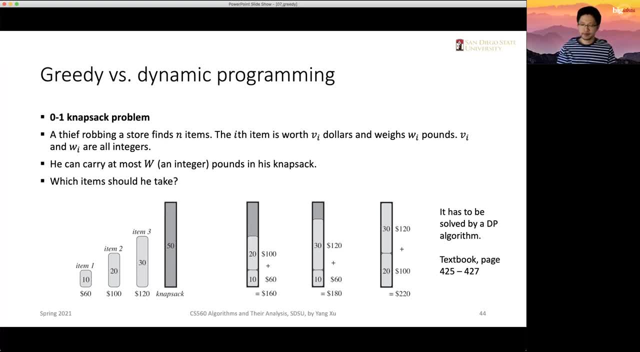 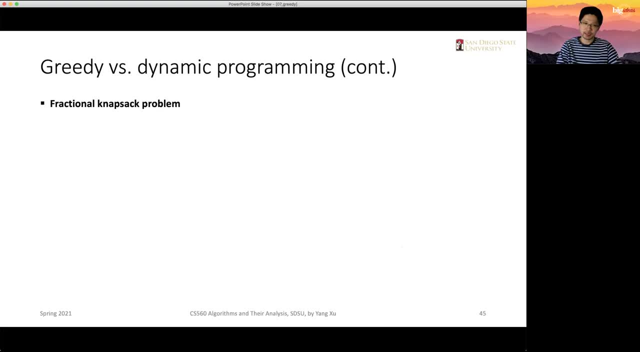 a little bit, then we will have a very easy, gritty algorithms solutions actually, and this is called- actually called a fractional knapsack problem. So the difference is that the thief can take actually fractions of the algorithm to solve the problem items. okay, it doesn't have to decide whether to take it or throw away one item. it's not like that. 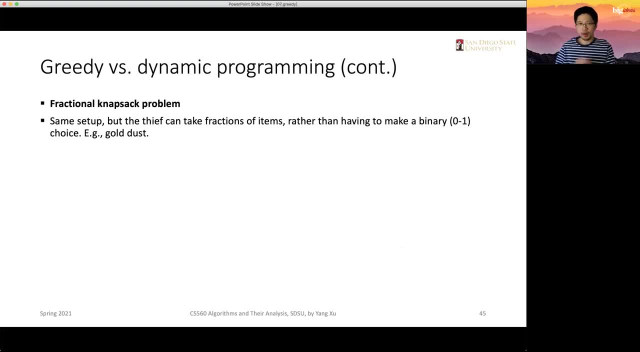 it's like you can have part of the object, part of the item, excuse me, like he has a gold dust right he can use, like pouring the dust into his knapsack as much as possible, like that, something like that. so it's called a fractional knapsack, so in this case it actually makes the 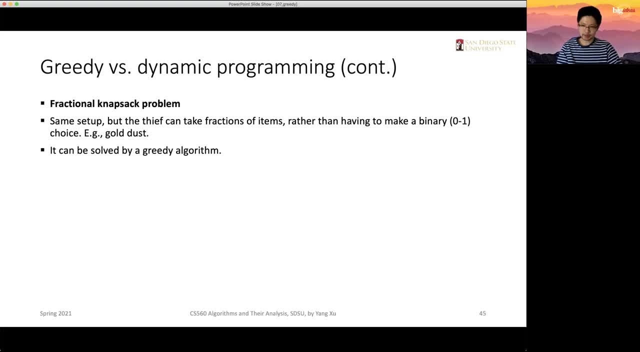 makes the problem quite straightforward to solve. okay, it's a very easy greedy algorithm thinking. it's like we can simply pick the most valuable item by looking at the rate, by looking at the ratio of value versus weight, right? so if that ratio is the highest, then we we say that this is the most valuable thing to to pick. 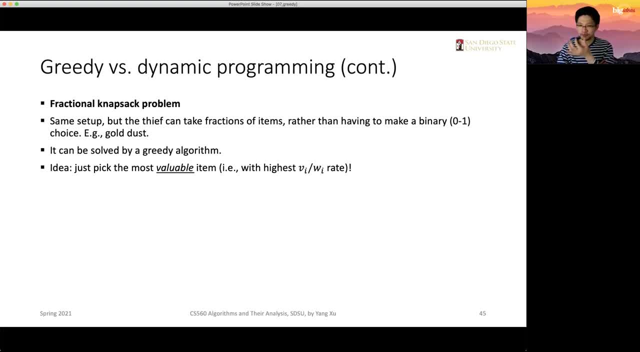 right, it's like the unit price, like the unit price for each items, because we can take a proportion of it like which, whatever proportion we would like. so that'll make the whole solution quite different. okay, so if you look at the unit price for each, for these three items, so these numbers, 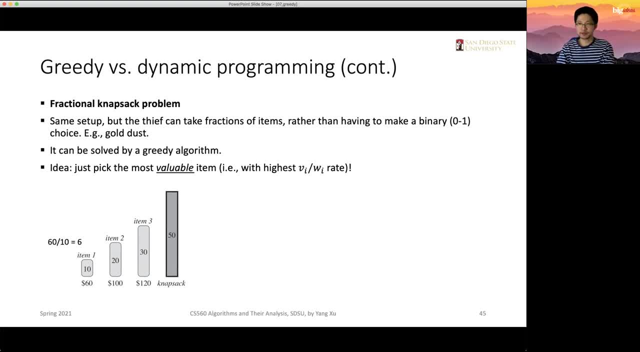 are the same from the previous slide, but but if you link off, think of the unit price. so for the first one it actually has 60 over 10, which is six, right. and the second one has a lower low unit price which is 100 over 20, which five. and actually the third, the item three. 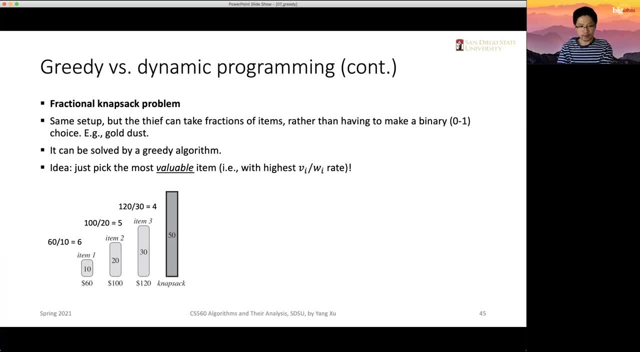 has the lowest unit price. okay, so according to our strategy, our greedy strategy, we want to take those objects that has the highest unit price right as much as possible. so the solution would be like: we will fill out the knapsack with these most valuable items first. right, that'll take up 30 pounds, and what we're gonna do with the next is that. 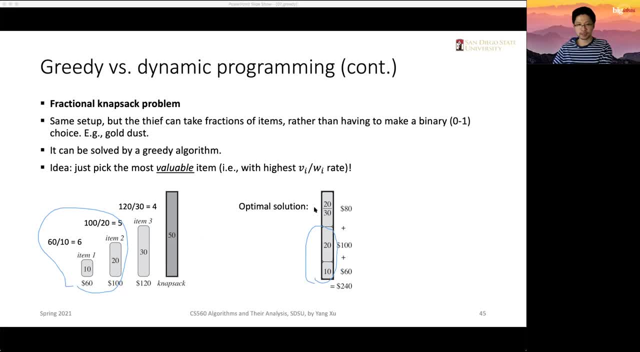 there are 20 pounds space left, right. we're gonna take that 20 over 30 proportion or fraction out of this item three. we only take the. we only take 20 pounds out of this. 120 dollars item three: okay, so that will be 60 plus 100 plus 80 dollars. okay, so that actually maximizes the, the solution. 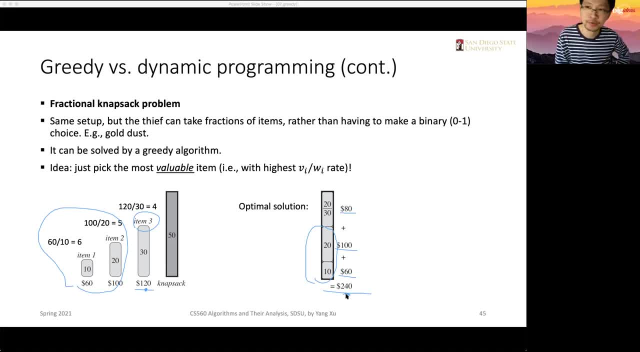 and it's even better compared with the previous zero or one knapsack problem. okay, so yeah, anyway, i hope this uh example makes the um showcase that the, the um, greedy algorithms, sometimes the the same problem can actually be converted into a totally different problem and, typically speaking, the, the, the. 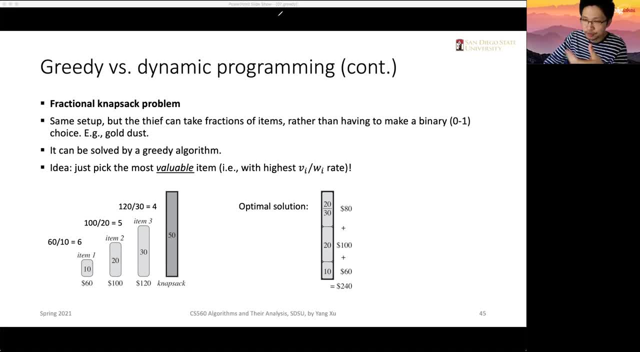 connection between these two different types of problems usually can be solved by the more complex one, can be solved by dynamic programming, while on the other hand, if we think of it in a different angle and change the condition a little bit, then it becomes a problem that can actually 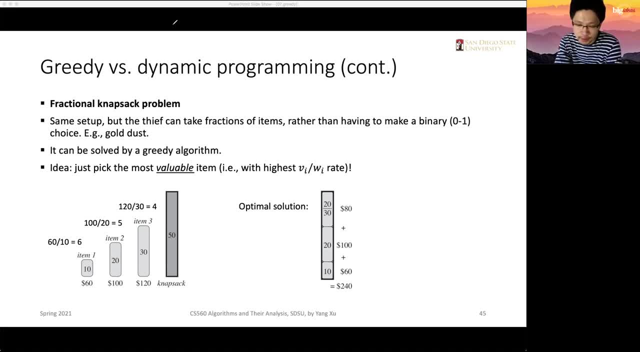 be solved with a greedy solution which is much easier to think about to come up with a solution, All right. so that's so much for the greedy algorithms today, and actually I don't have more slides today, so I will end the class a little bit earlier. and the algorithm? oh no, the assignments for the. 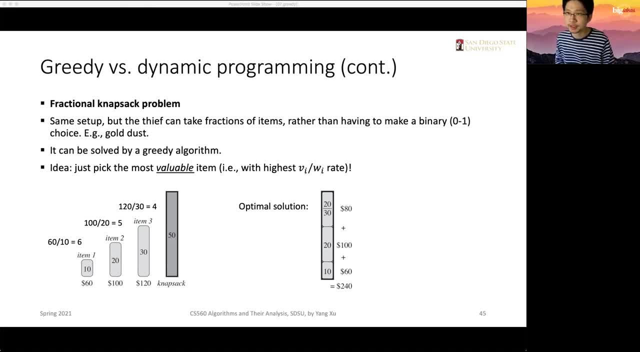 greedy algorithms. I will release it this evening later or later this evening tonight. okay, so it will be like several problems you can work on about the activity selection, about the Huffman codes and some other types of problems That can be solved from a greedy selection, from a greedy choice perspective. okay. 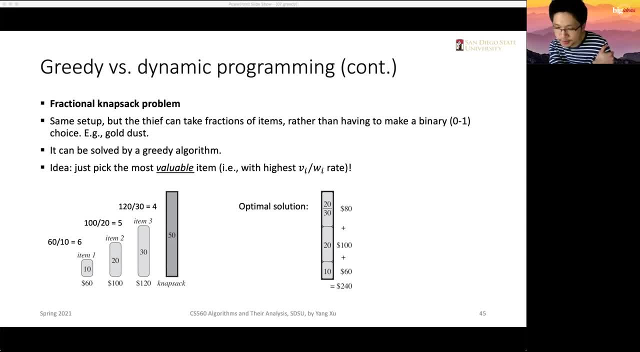 Yes, professor. yes, regarding the current assignment, the one about dynamic programming, I recall earlier on you said it would be due this Friday, but the Canvas says it's due the 23rd. Yeah, yeah, I extended that. Okay.